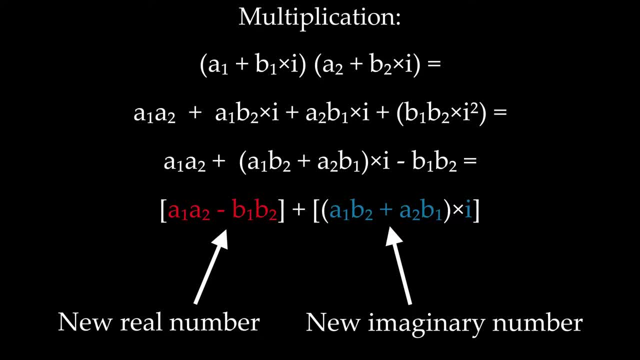 components of the two complex numbers. When multiplying or dividing any amount of complex numbers, if we encounter i squared or i to an integer power that happens to be of the form 2 plus a multiple of 4, we simply change it to negative 1.. 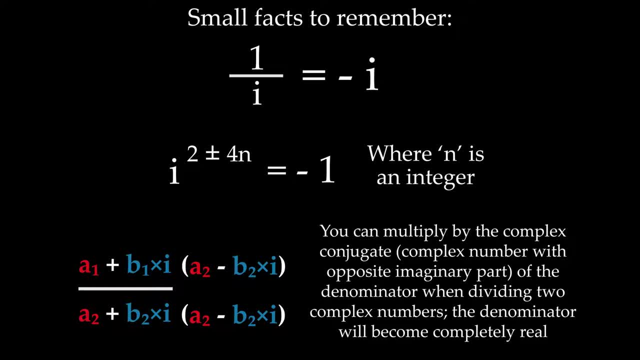 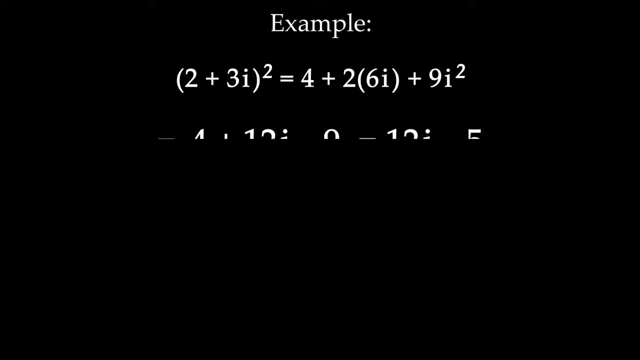 Here's an example of a complex number that can be divided by a real number. Since we just squared the number, and z squared is a function, it would make sense that there would be a way to visualize this function for a set of inputs. Before we get to that, though, I want to go. 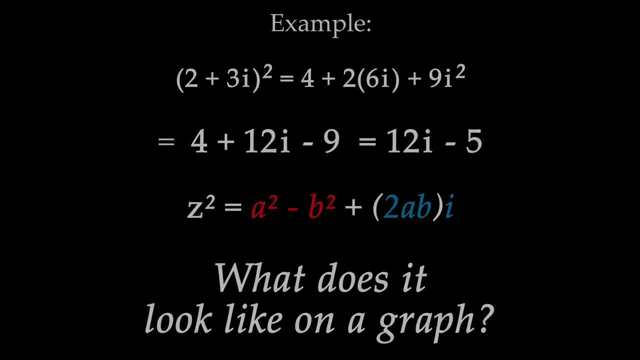 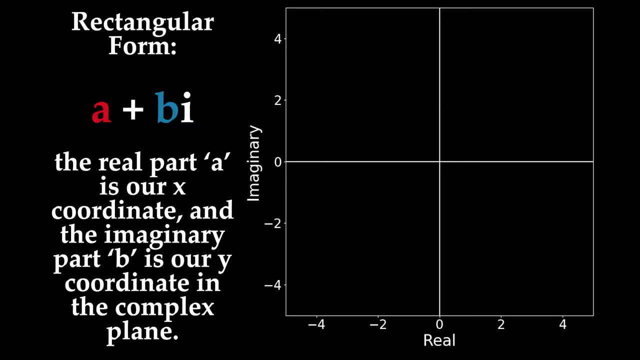 over the two ways to express a complex number graphically. One way to represent a complex number is using rectangular form, also called standard form. Here we have a graph representing the complex plane of a complex number. We can see that the complex plane of a complex number is a. 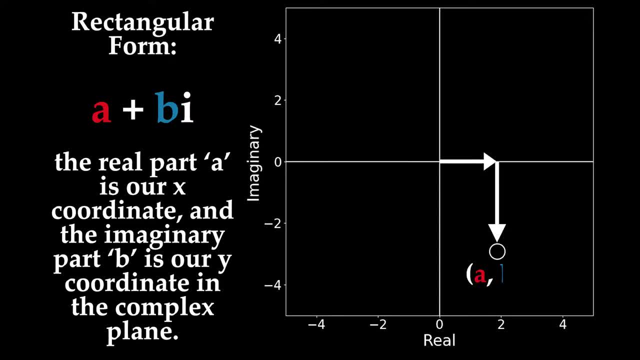 plane which contains all the complex numbers. On this graph of the complex plane, the real part of each complex number is determined by its horizontal coordinate. The imaginary part of each complex number is determined by its vertical coordinate. A second way we can represent a complex number is 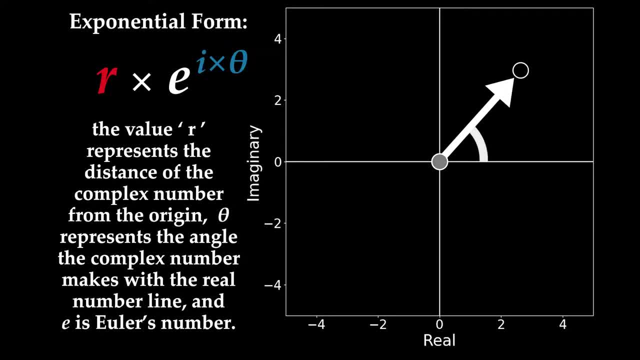 using exponential form. Any complex number can be written in the form: r times e to the power of i times theta. It's not really obvious why e would show up here, so I've included a link in the description to a proof of why a complex number can be written like this In this form. r represents. 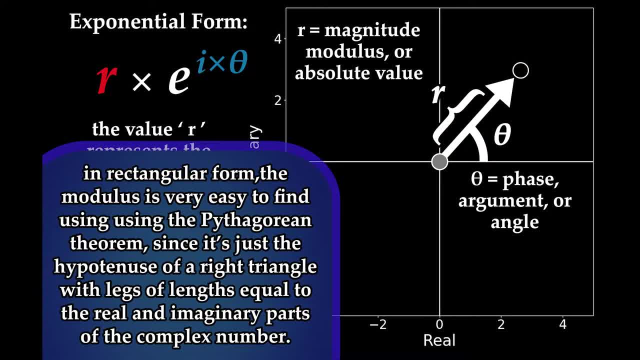 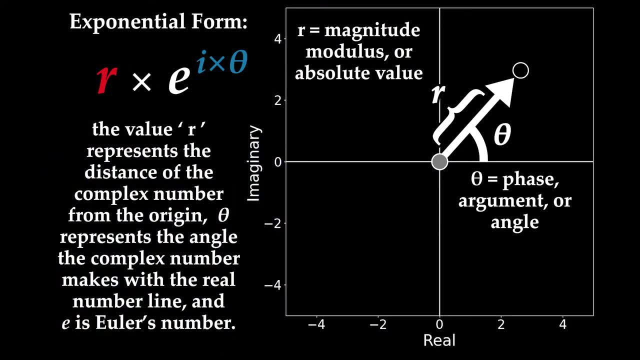 the distance that the complex number is from the origin of the graph. This distance is called the magnitude modulus or the absolute value of the complex number. The angle theta represents the angle that the complex number makes with the real number line. This angle is called the phase or the. 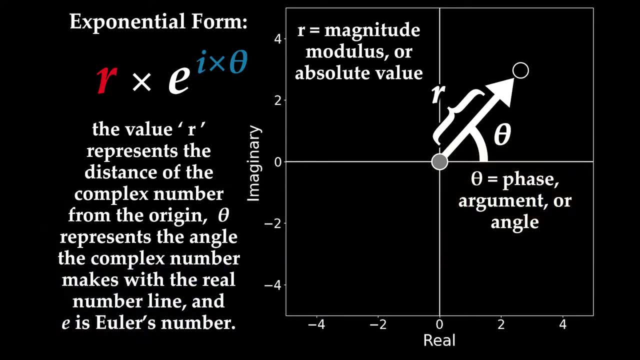 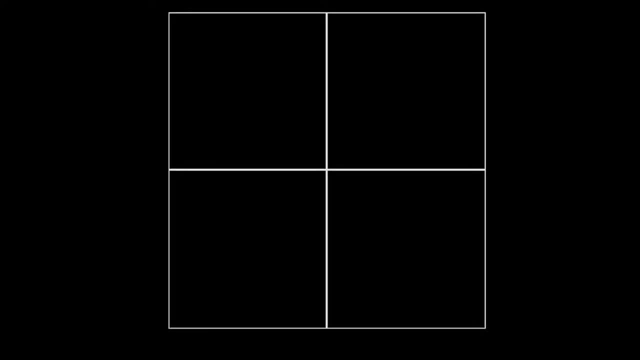 argument of the complex number. It can be very convenient to write a complex number like this in a lot of scenarios. There's a lot of ways to express a complex number graphically and the. there's one more thing I want to point out, Since complex numbers are two-dimensional. 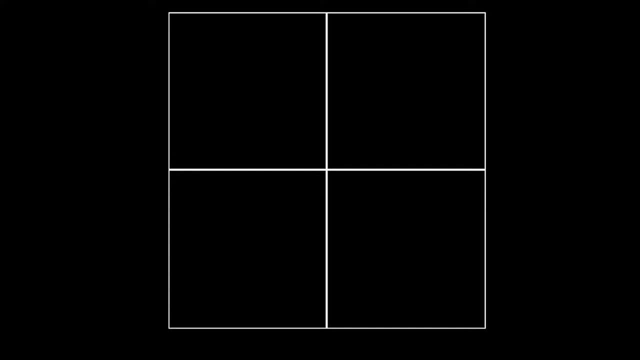 having distinct real and imaginary components, our input isn't going to be restricted to a single one-dimensional line, like it would be for a completely real-valued function. In the case of a complex-valued function, the input can be any two-dimensional shape, and so can the output. 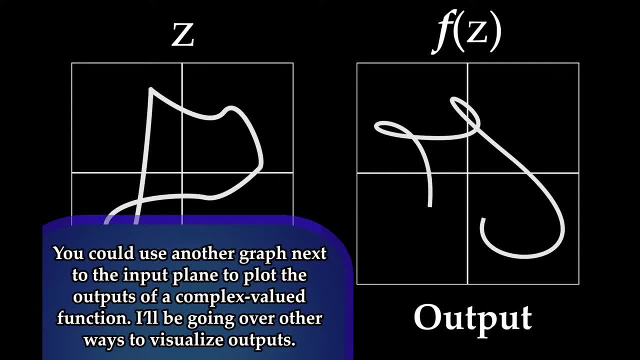 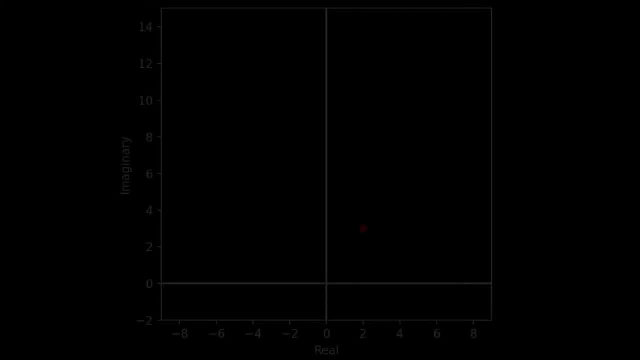 To start, let's consider the example point from earlier: 2 plus 3i. We'll square the point and see where it goes. We should expect it to go to negative: 5 plus 12i. Since there's only a point to be drawn on the free hand, we can set the value of 0.5.. 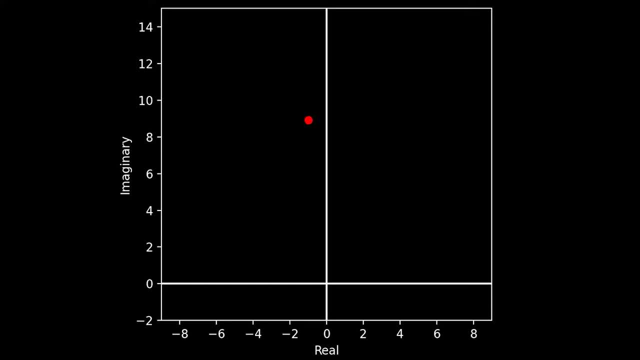 We can alsoヽ set the value of 0 and try the problem with that value. So let's perform that first. Let's try the example on the right. We should be able to do that on the free hand, but it's hard to predict where it will go. We should expect it to go to negative 5.. 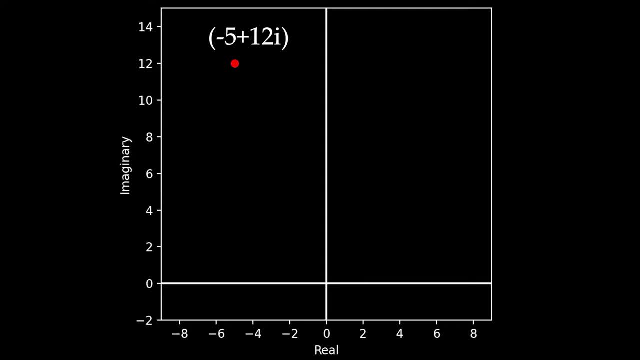 Since there's only a single point associated with the square of this complex number, you may be wondering whether this motion of the point was arbitrary. We should expect a single jump to its square, as opposed to a smooth movement. The path wasn't arbitrary, though. 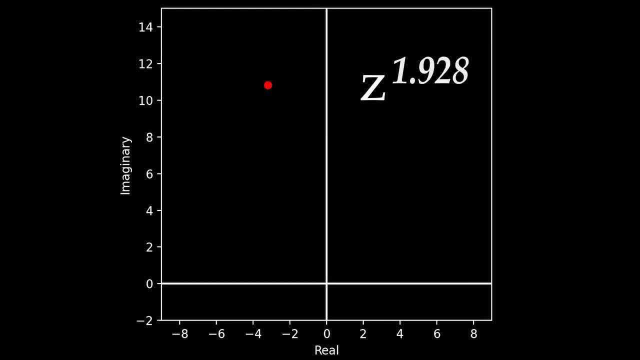 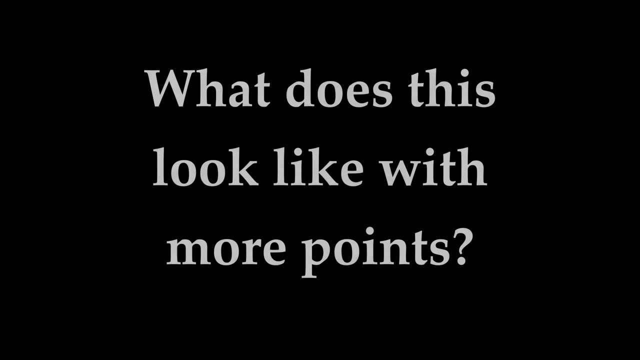 What this animation shows is actually the exponent of the function z to the power of k, changing continuously and stopping at z squared. This is the particular path that the point follows to its square when the exponent changes in this manner. Obviously, here we're only seeing the animation for one point, so to get a better idea of 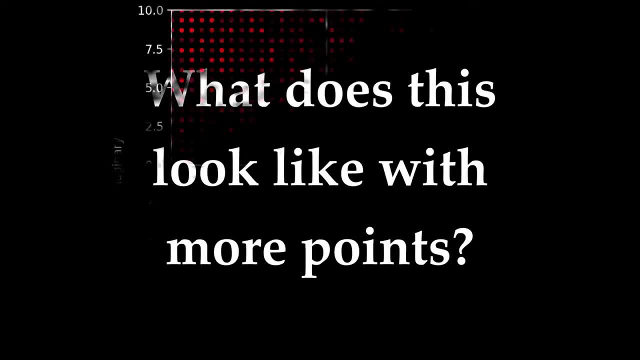 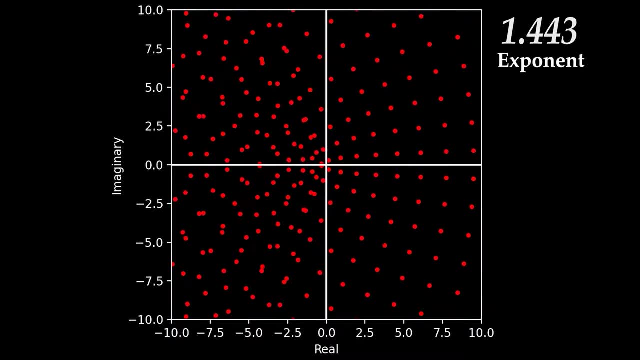 what happens to an entire piece of the plane. when we apply this function, we can look at a grid of points. At z squared we see this symmetrical distribution of the points. Obviously, these points are the ones that would map back to a square grid if we took their. 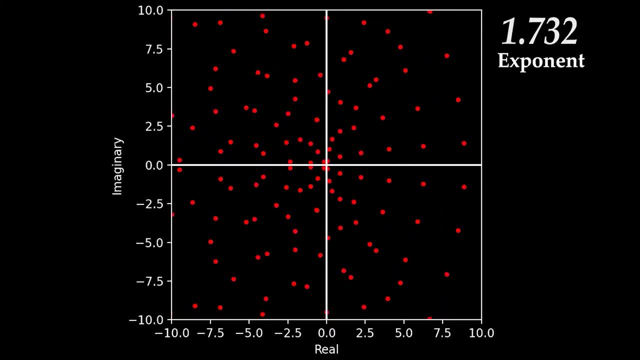 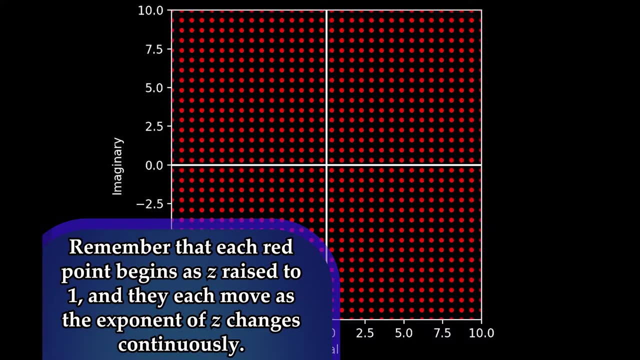 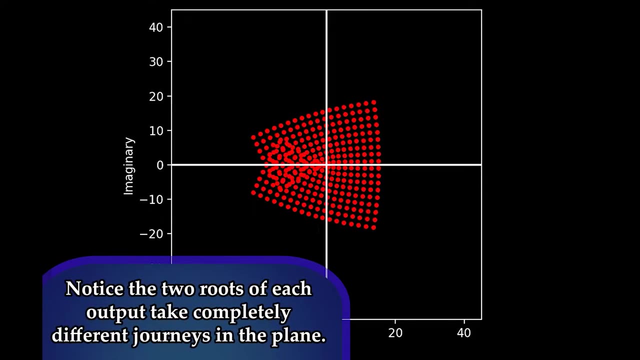 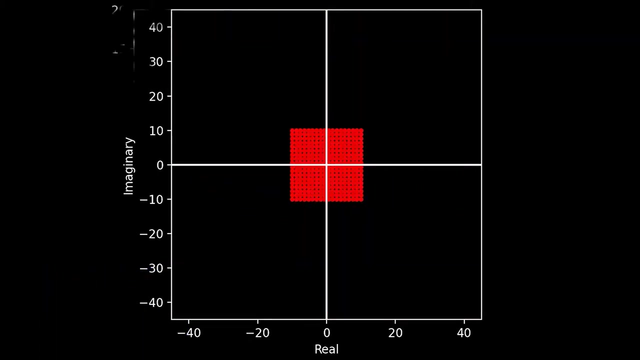 square root, though it would be hard to tell this if we didn't already know. Okay, Let's zoom out even more. we can see that the grid seems to fold in on itself during the transformation from z to z squared. Here's what it looks like if the exponent goes beyond 2 in the animation. 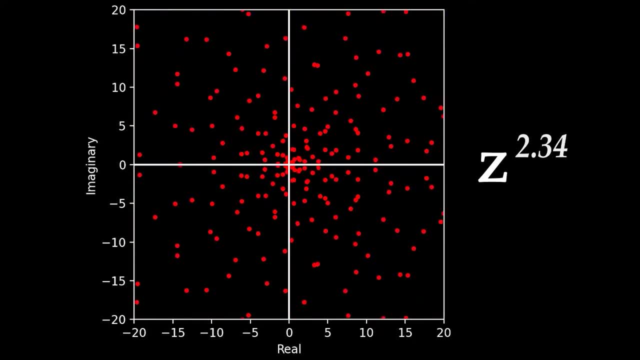 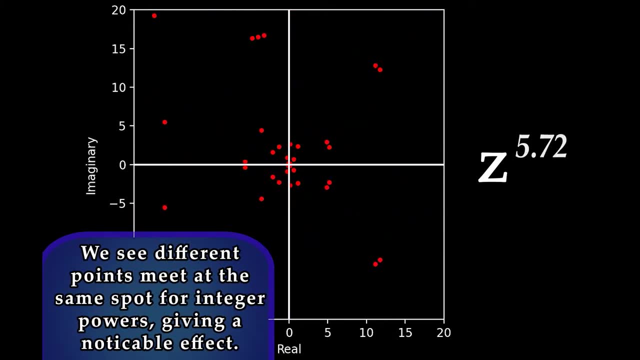 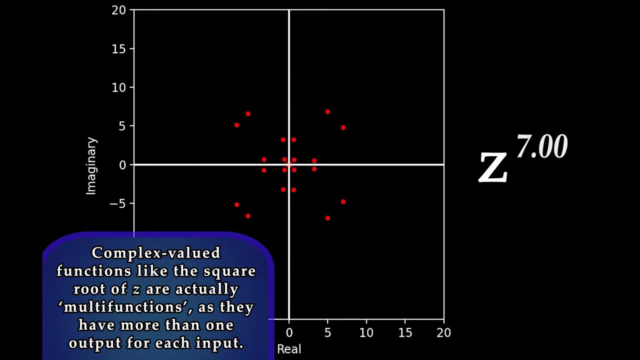 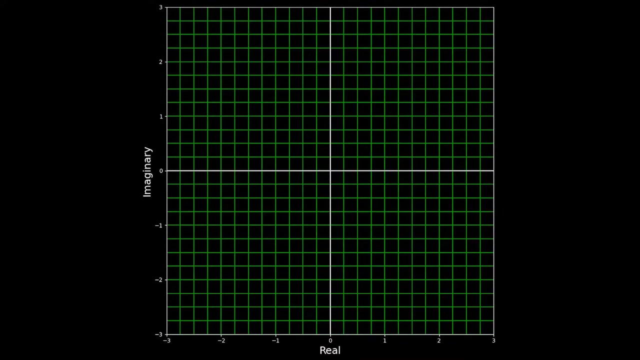 Here's what it looks like if the exponent goes beyond 2 in the animation, Instead of using discrete points, we can use continuous lines to represent the inputs and outputs of a transformation in the plane. At the beginning of the video, the image labeled conformal map shows what a square grid of 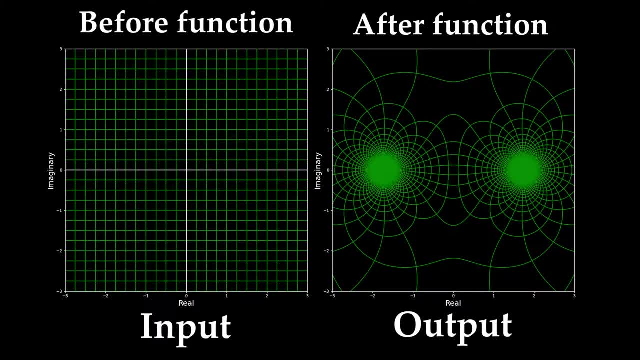 continuous lines would transform to if passed through the function z over the quantity z squared minus 1.. Here's what the grads of this equation's lines would show us if they passed through the function z over the quantity z squared minus 1.. 3. A conformal map is essentially just a function in the complex plane that leaves the angle between: 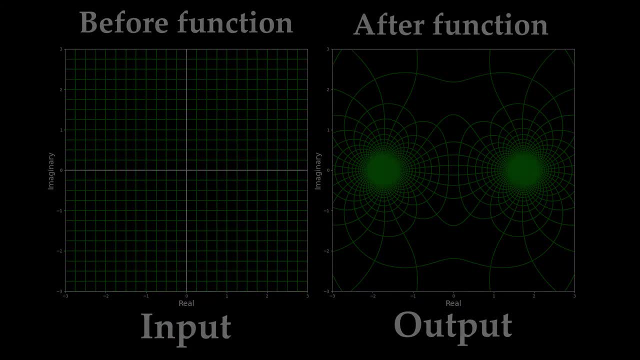 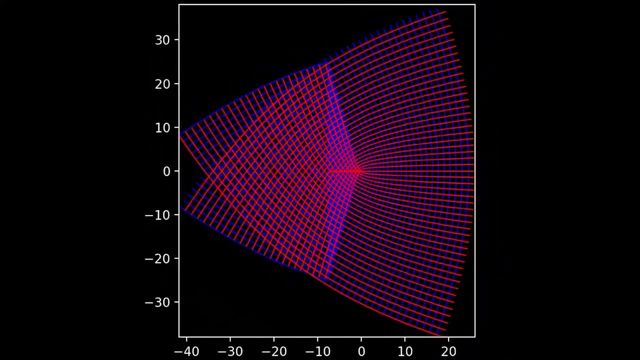 the intersections of continuous gridlines in the plane unchanged after the transformation occurs. For example, if we start out with a grid of lines which intersect each other at 90 degree angles, then after a conformal mapping is applied, the angles at the intersections will still be 90. 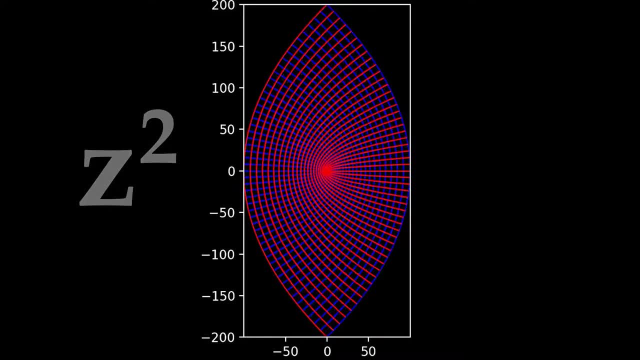 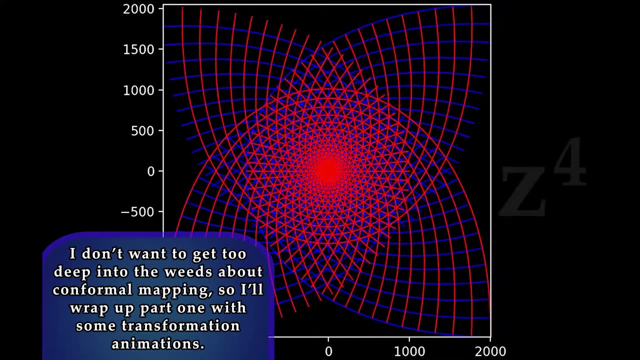 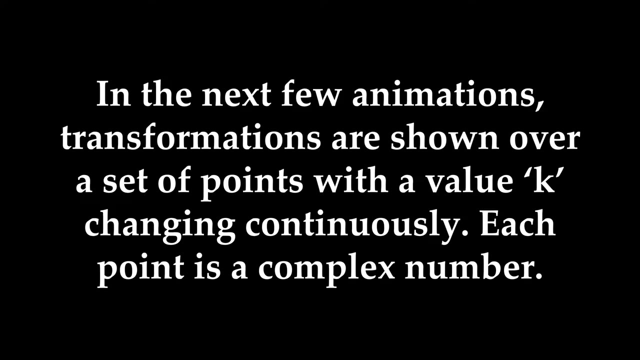 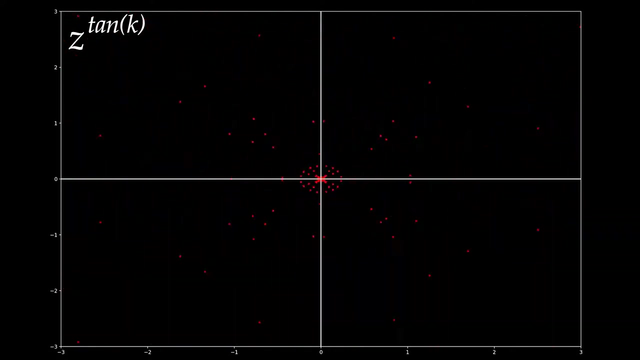 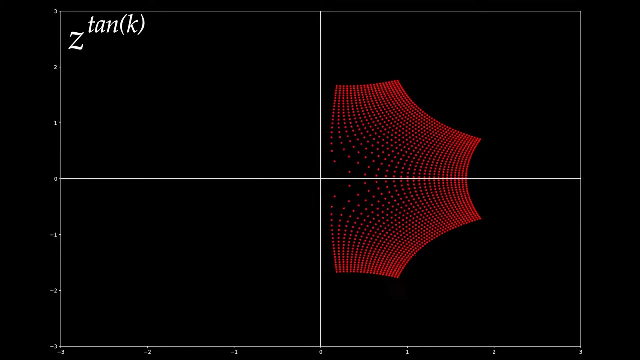 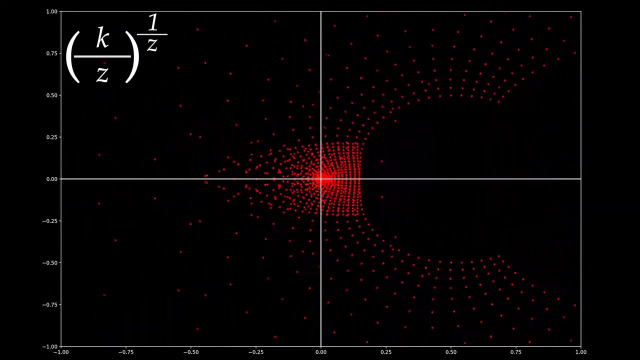 degrees. A function must be complex, differentiable or what's called holomorphic on a set of points in order for it to be a conformal map on that set of points. A conformal map is a set of points in order for it to be a conformal map. 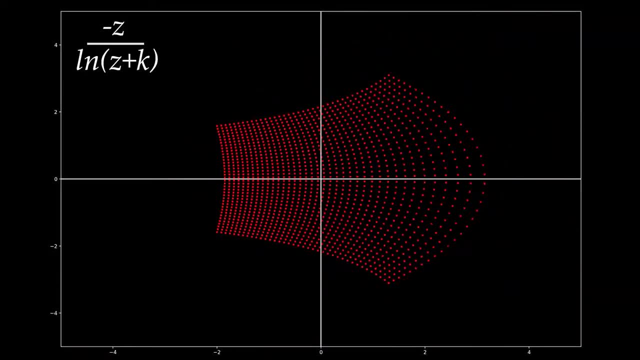 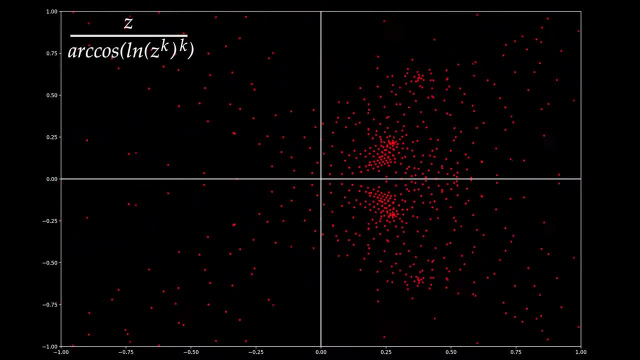 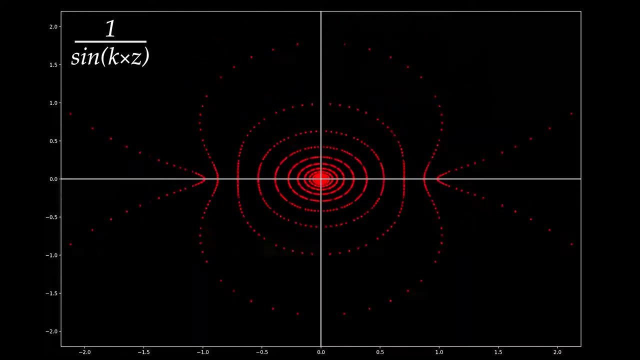 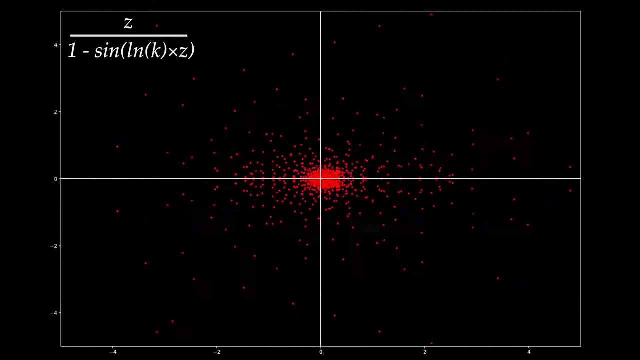 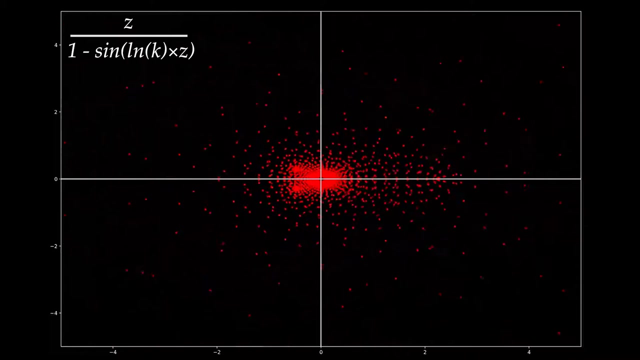 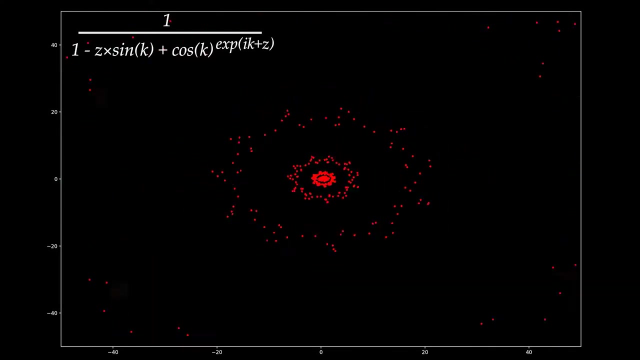 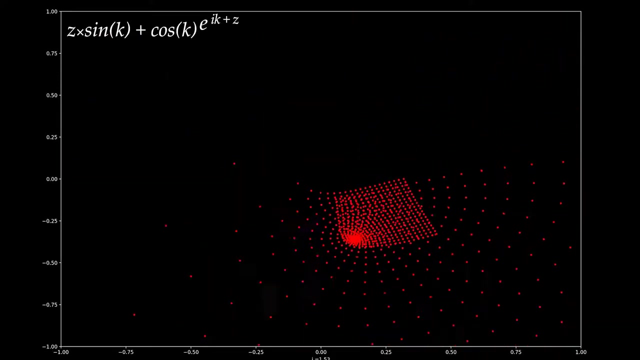 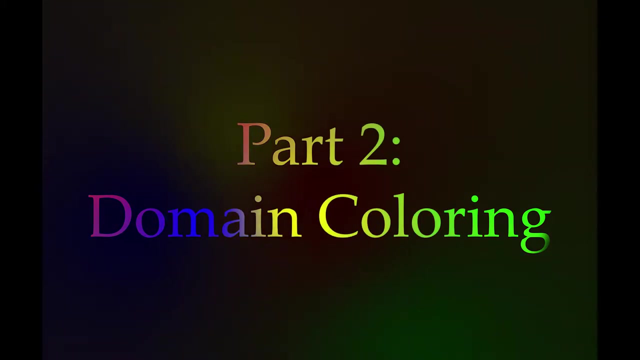 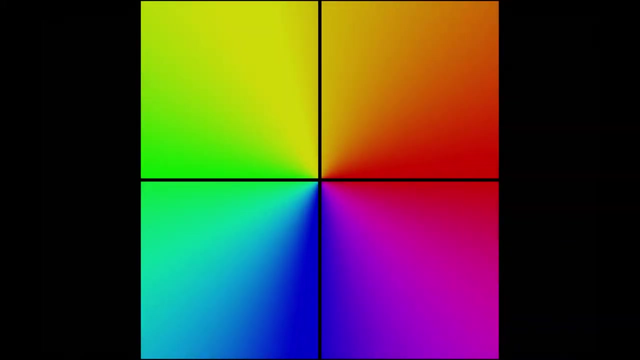 A conformal map is a set of points in order for it to be a conformal map. As the name implies, domain coloring is a technique that we can use to visualize the outputs of a function or transformation in the complex plane using color. As the name implies, domain coloring is a technique that we can use to visualize the outputs of a function or transformation in the complex plane using color. 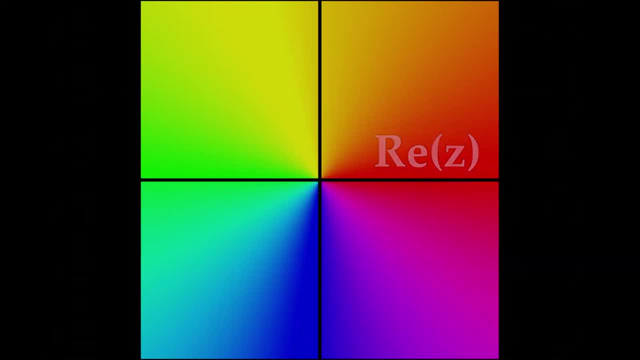 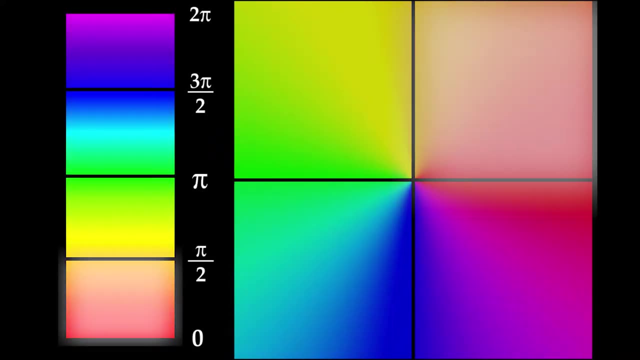 Here again we have our real and imaginary axes. The color represents the phase of the complex number. Every complex number is assigned a color based on the angle it makes with the real number line. This particular graph simply shows the unaltered complex plane. 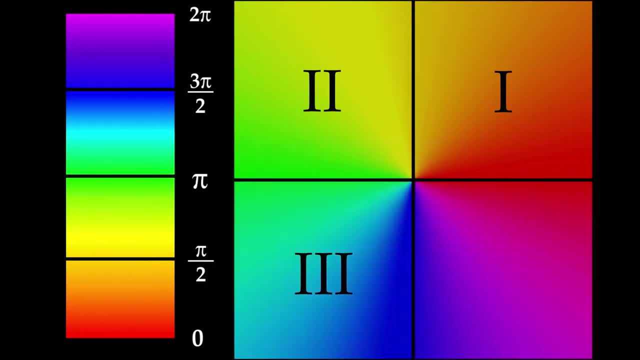 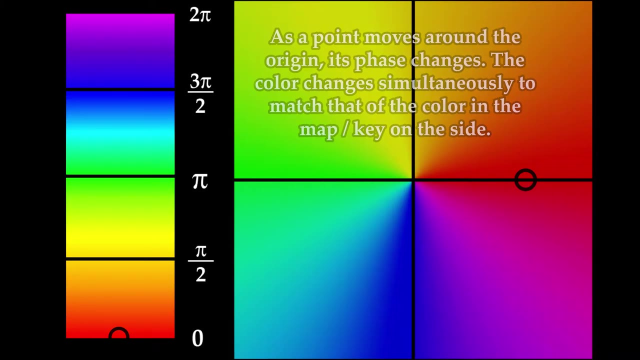 This way, we can see which color is associated with which part of the plane. Using a color map on the side, we can match the color of the output to its corresponding phase. Enable yourniks. If the moment with which the first part of a piece is desired is arrived, then the second part of the segment, bizimawiz. 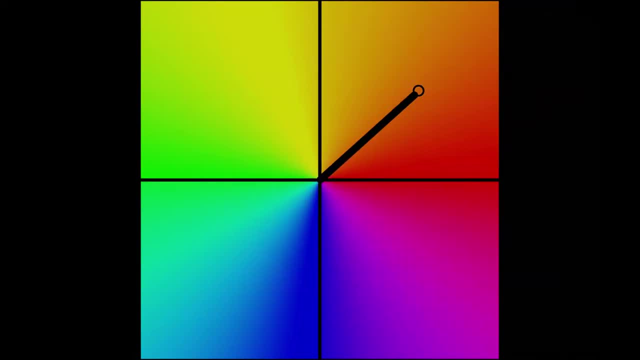 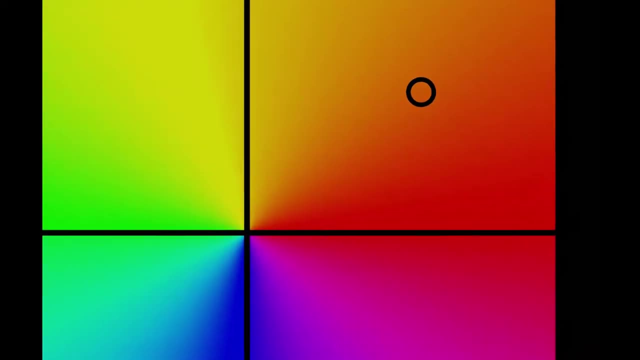 is directly preceded by the base element. Let's say a complex number has a phase of 42°. Let's say a complex number has a phase of 42°. By just looking at the color at this point we can determine from the color map that the phase of the output at this point is roughly π over four radians. If the color at the output at this point is roughly π over four radians. If the color at the output at this point is roughly π over four radians. If the color at the output at this point is roughly π over four radians. 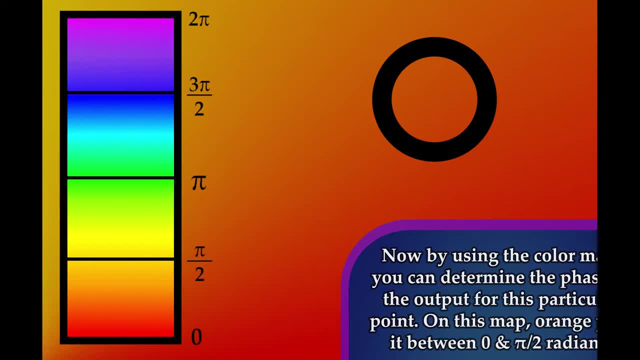 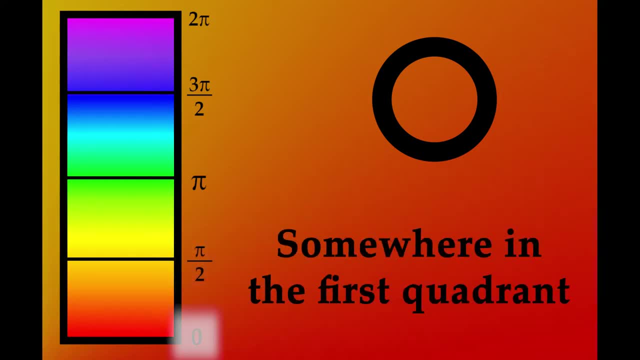 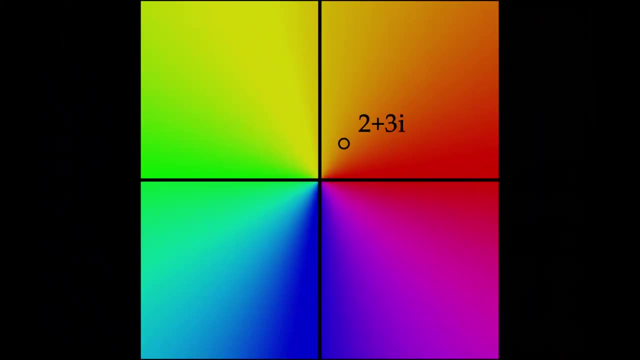 radians, or about 45 degrees, which is pretty close to the actual phase. Before we see what happens to the entire graph when we apply the function z squared to the plane, consider again the point 2 plus 3i. The square of this point negative 5 plus 12i. 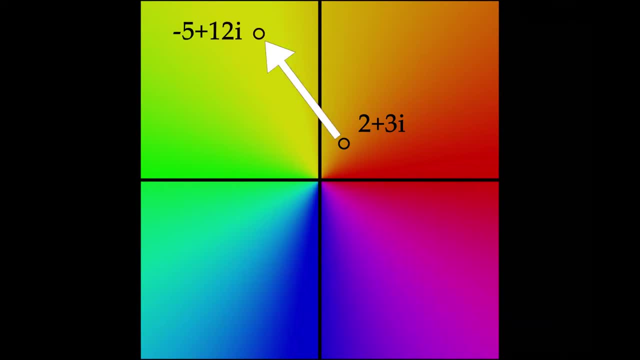 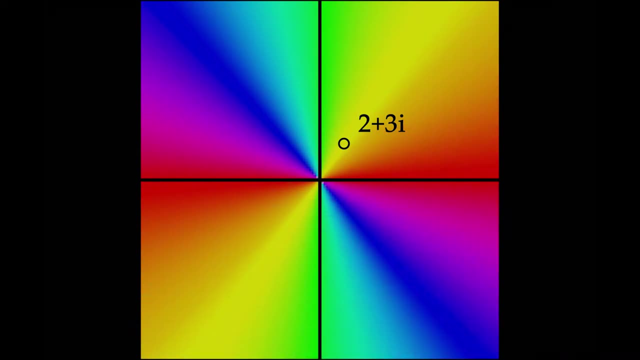 lies in the yellow region of our unaltered complex plane. Keep in mind this color. Now, if we square all the points in the graph, we get this. Now look at the location of 2 plus 3i. The color at this point is yellow. 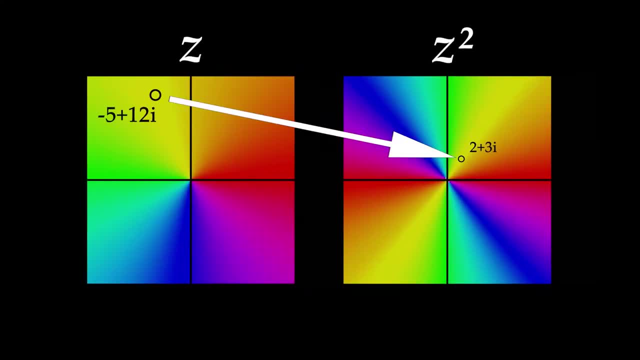 just like the color of its square in the first graph of the unaltered complex plane. From this we can deduce that the phase of the output for this point corresponds with the color yellow. As long as we have a key for matching color with argument, we can roughly determine. 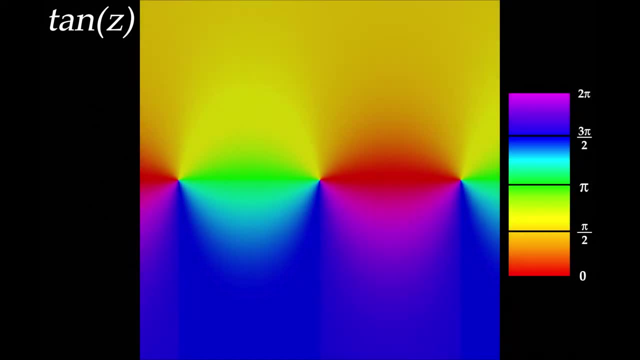 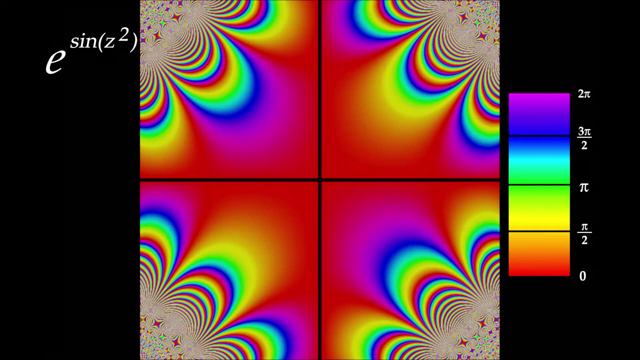 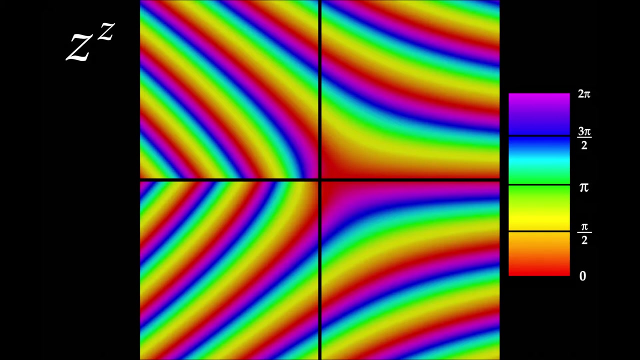 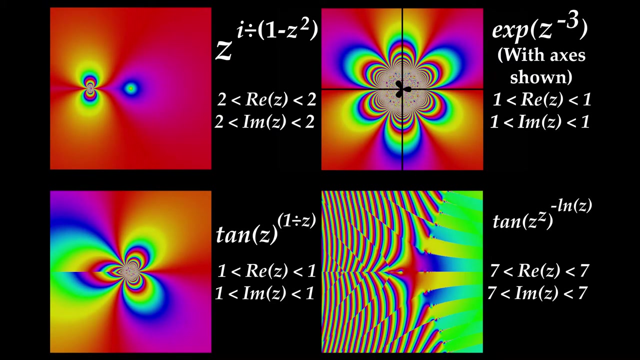 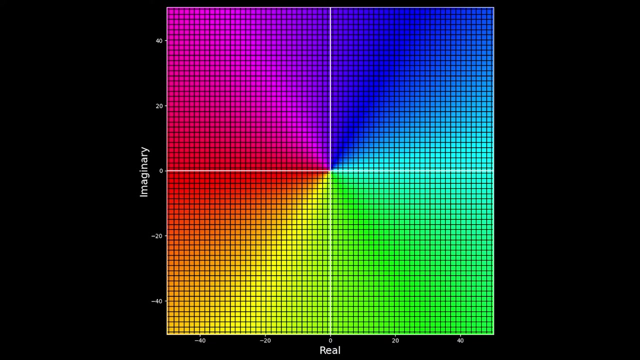 the phase of any output in the image. Here are some more examples of domain coloring. One thing you can do to get even more information about a transformation is superimpose continuous lines on top of a colored image of the plane. This simultaneously shows how a transformation 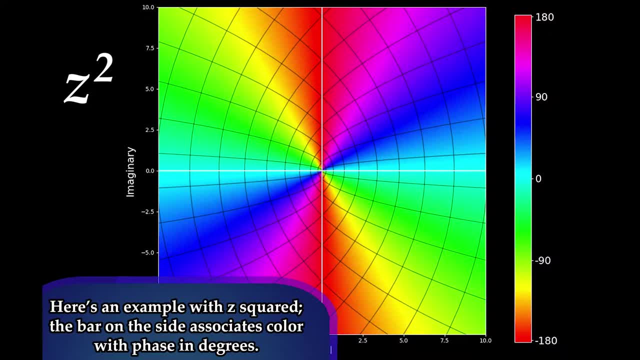 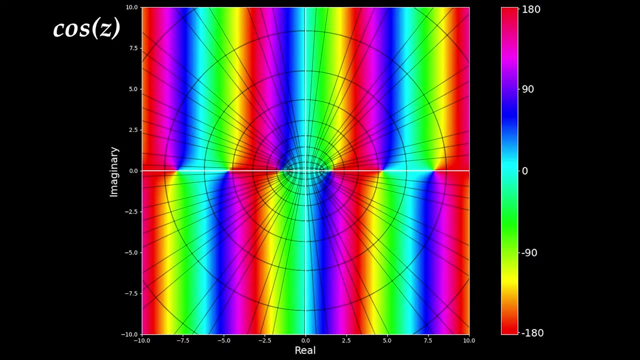 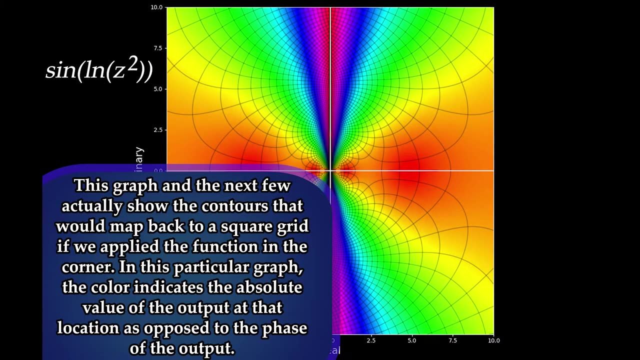 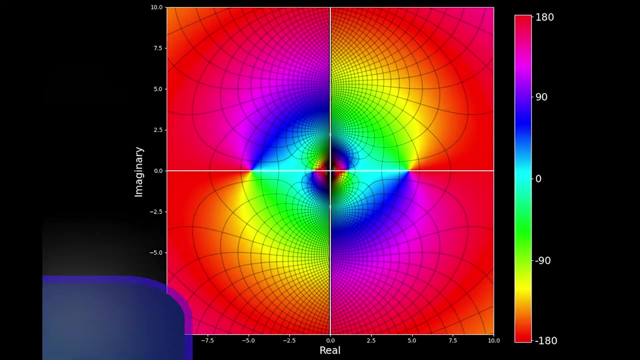 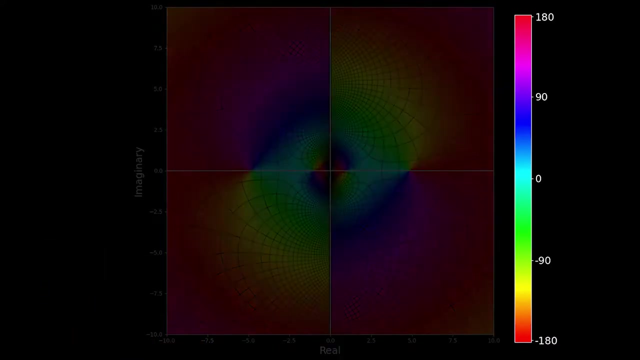 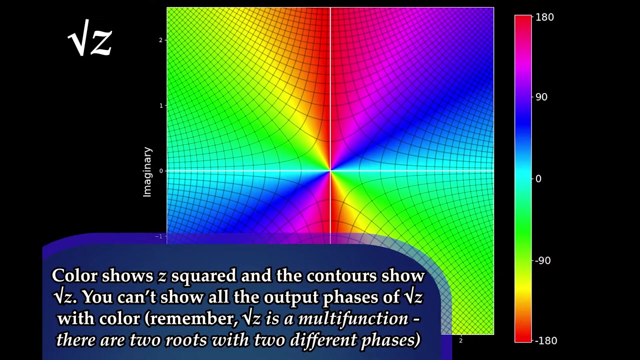 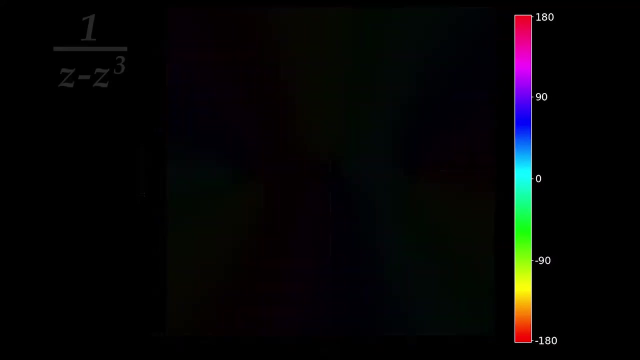 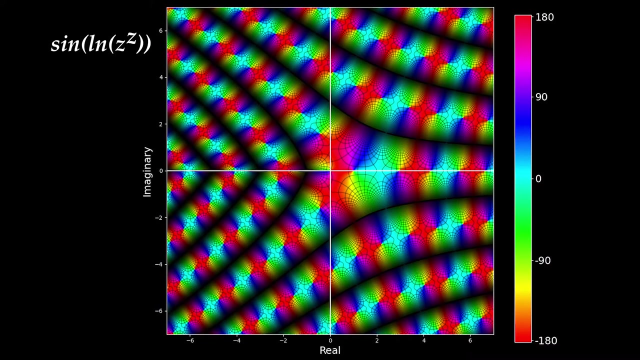 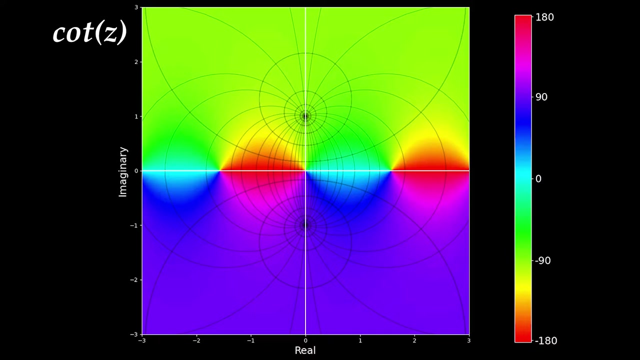 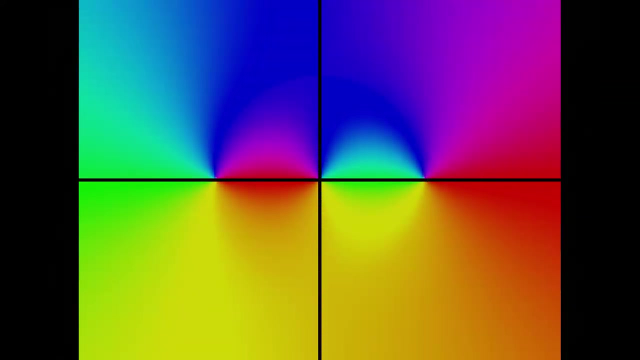 warps gridlines in the plane and how a transformation warps gridlines in the plane and how the transformation affects phase. I hope you enjoyed this video. We'll see you next time. Here's the colored plot for the function z over the quantity z squared minus 3, the 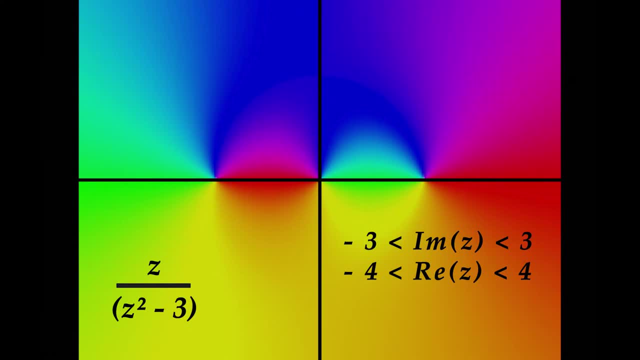 function from the beginning of the video. From this image, we can determine the phase of our outputs, but not the absolute value. In order to visualize the absolute value of the outputs for this function, one thing we can do is utilize the third spatial dimension. 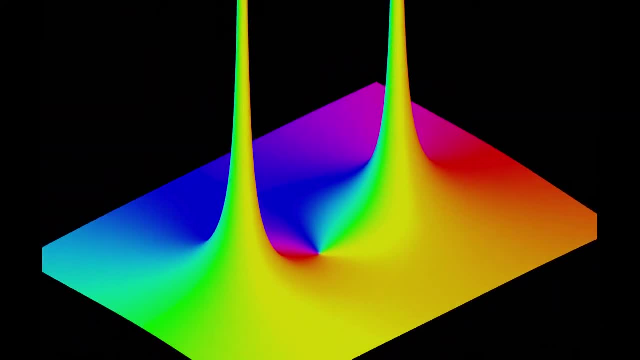 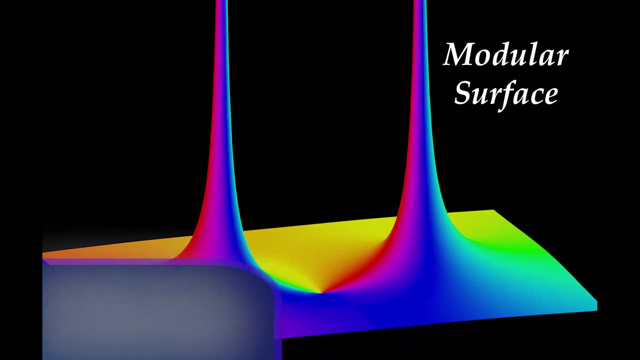 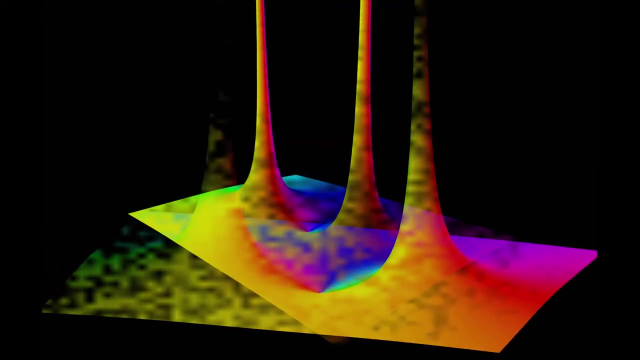 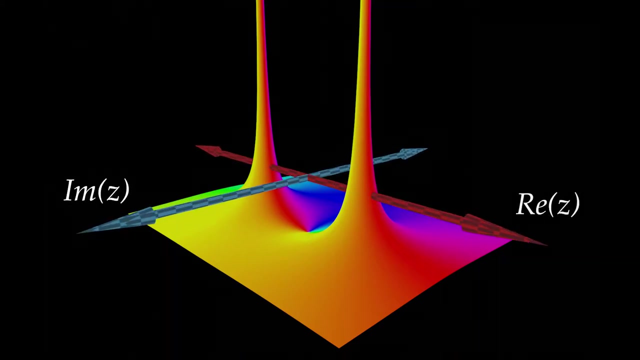 Now the z-axis represents the absolute value of the outputs. This representation of the outputs is called a modular surface, and these spikes around the undefined points in the plot are called poles. Close to the undefined points, the denominator of the function becomes extremely small. 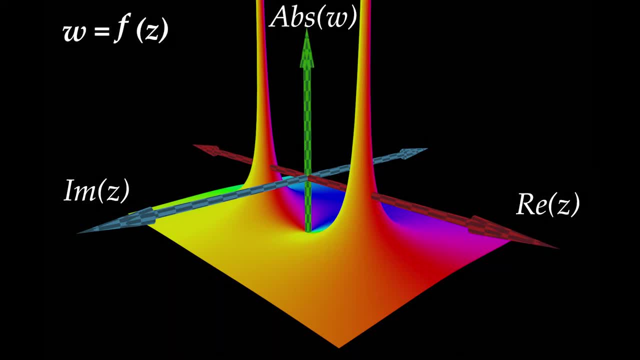 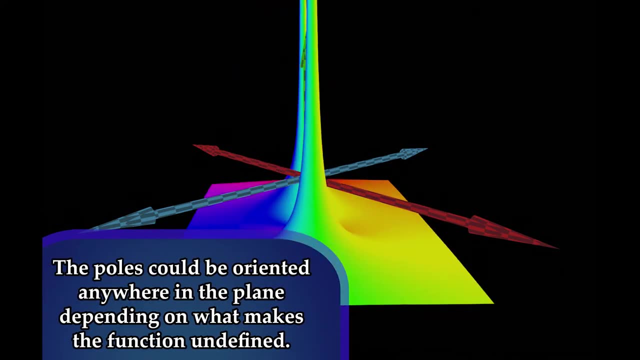 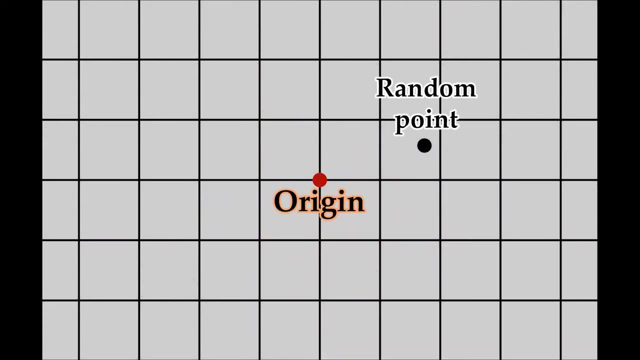 Regardless of which direction we approach, plus or minus, the square root of 3 from the output will tend toward infinity. To make sure that this makes sense, let's go over how to determine the output of a random point in the plane using a colored modular surface. 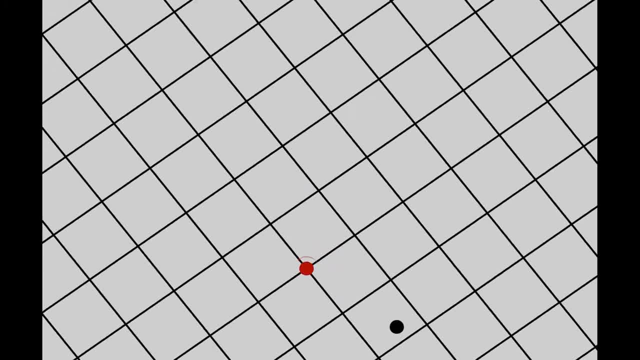 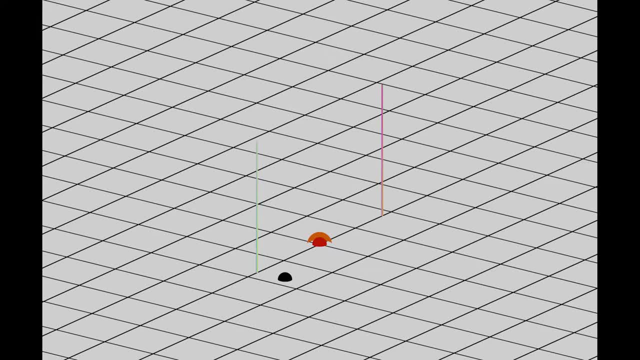 This flat plane represents our input space. Each complex number we use as an input can be described by a position on this flat plane. Now that the added spatial dimension represents the modulus of the output, we can interpret a distance from the origin along the z-axis as how far the output lies from the origin. 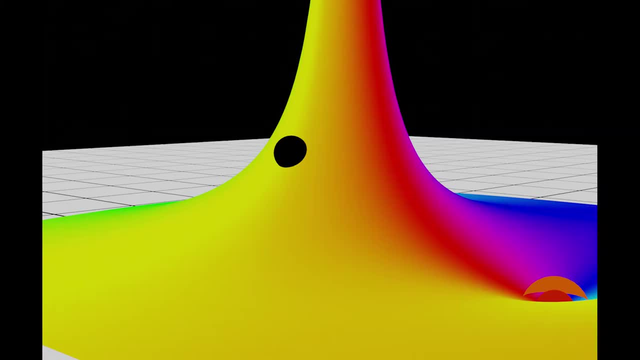 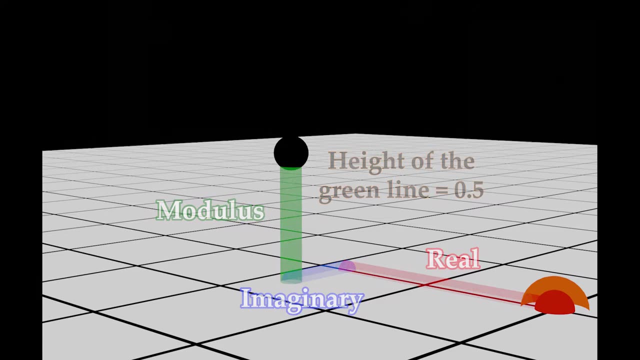 of the complex plane. Let's say that the height of this point on the surface is 0.5.. That means that the modulus of the output for this point is 0.5.. To find the phase of the output for this point, we can just look at the color at the point. 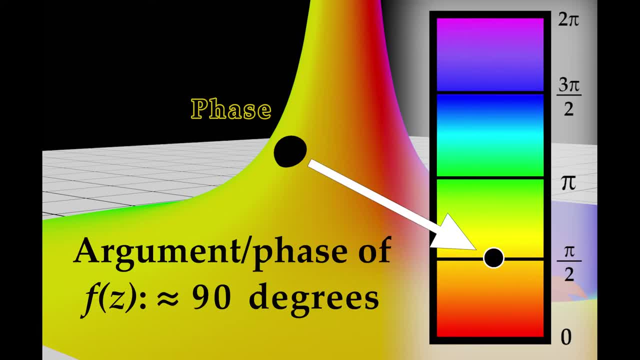 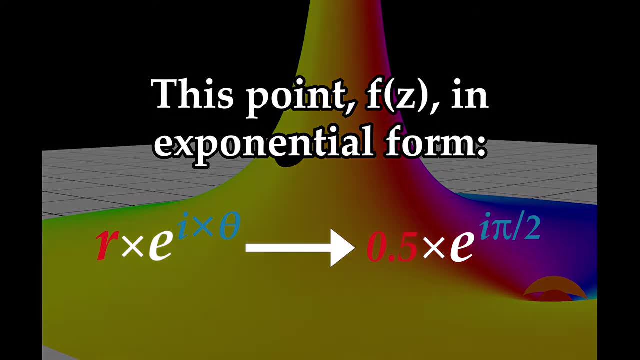 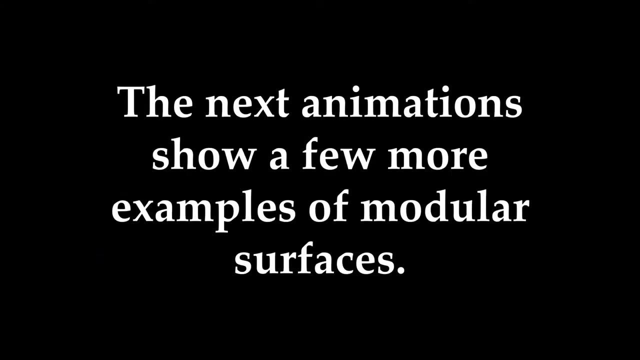 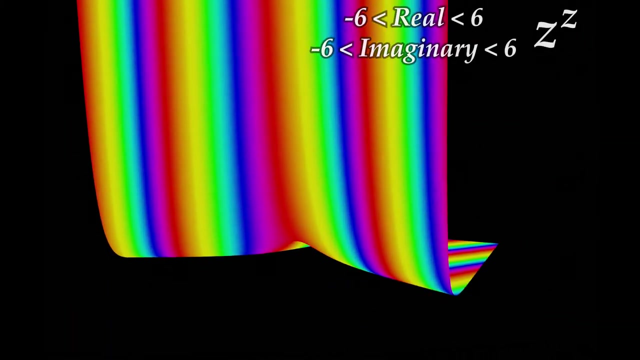 on the surface. Putting it all together, we find that the output of this point is about 0.5 times e to the power of i times pi over 2.. We should then push the value warehouse up to 1.. Now the value warehouse of the Predzieć vector A will be greater than or equal to the value. 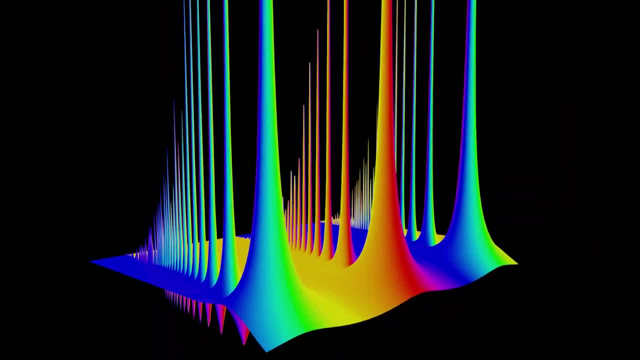 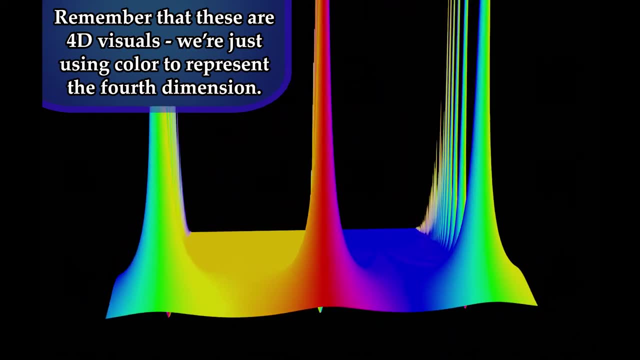 warehouse of z-axis, The value warehouse in for each of these three vectors is equal to 0.5.. If we look at the velocity of the 자꾸 plane, which is created by moving in and out of this view efficient, we can see that theться in the classroom, at the point e plus m, is asleep. 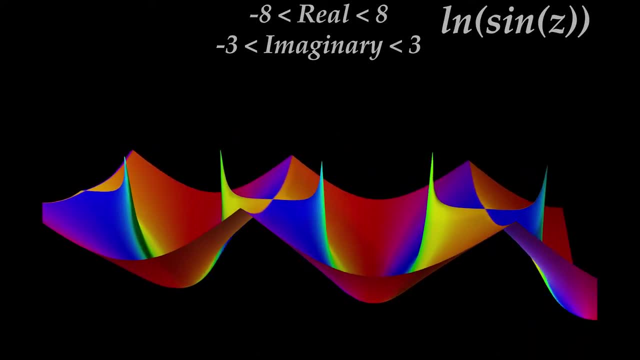 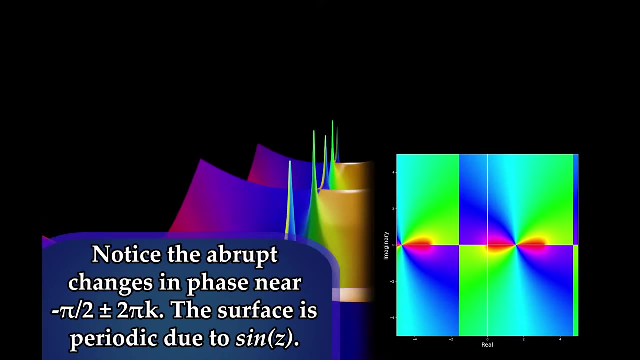 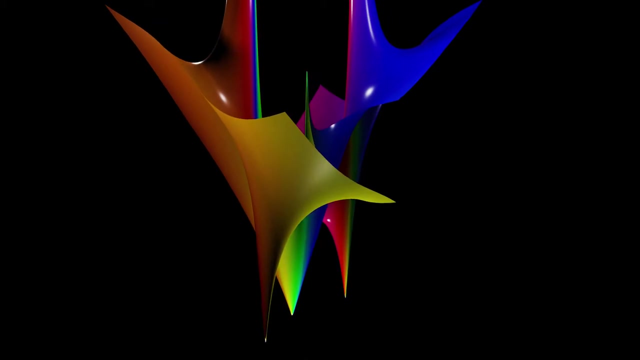 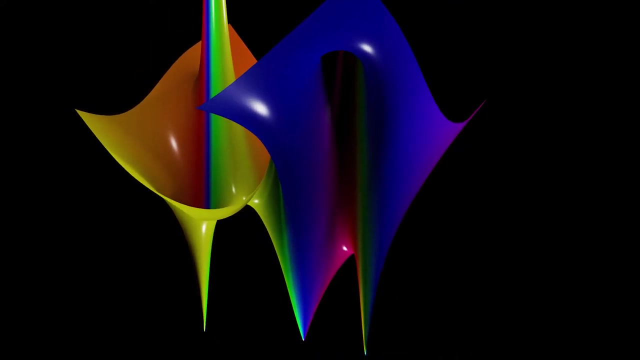 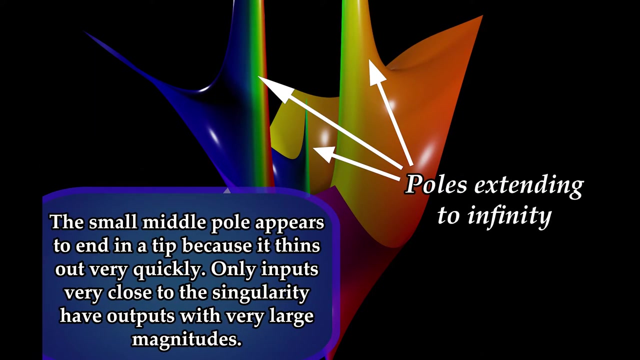 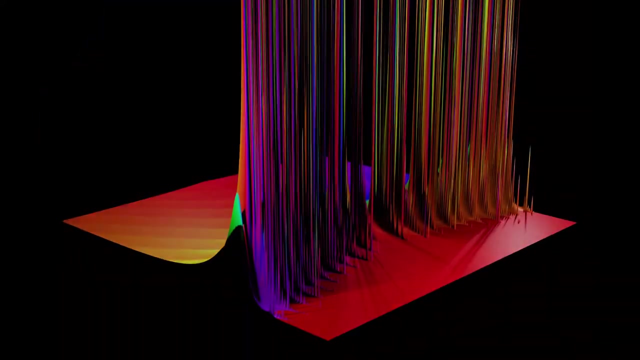 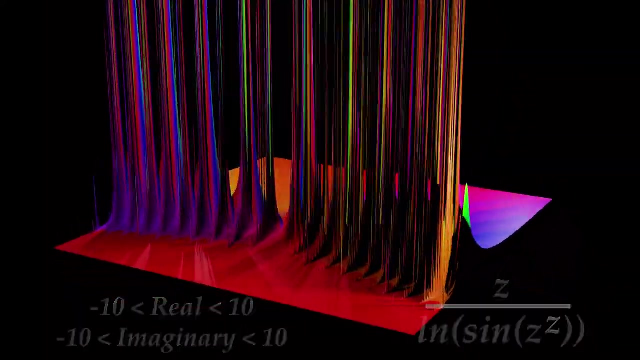 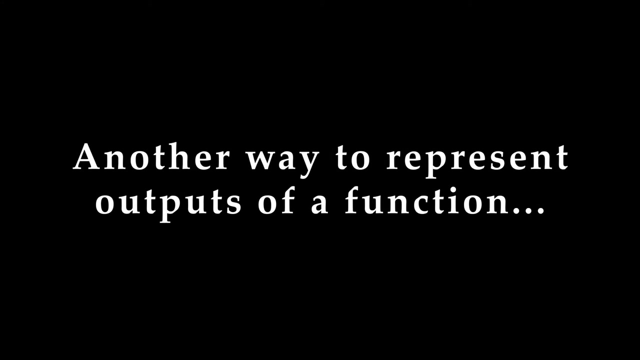 Therefore, we have an energy- contributivity series. Let's take a look at our already explained cinematics- laterok instruction. Thank you, There's one more way to visualize the outputs of a function that I want to talk about. If, instead of letting the third dimension represent the modulus of the output, 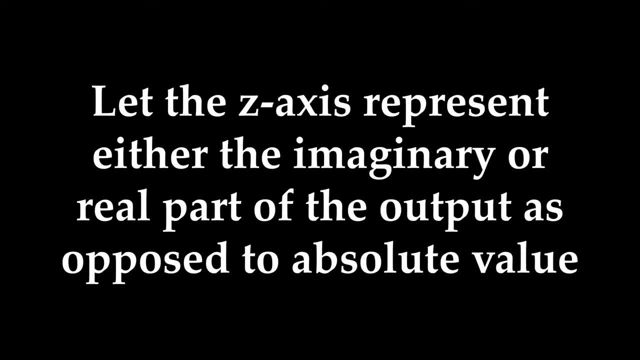 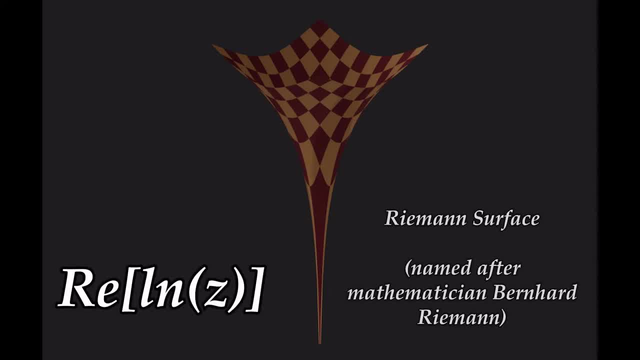 we can let it represent the real or imaginary part of the output. This is called a Riemann surface. As an example, this image shows the real part of the output of the natural logarithm of z near the origin. As we approach the origin on our input. 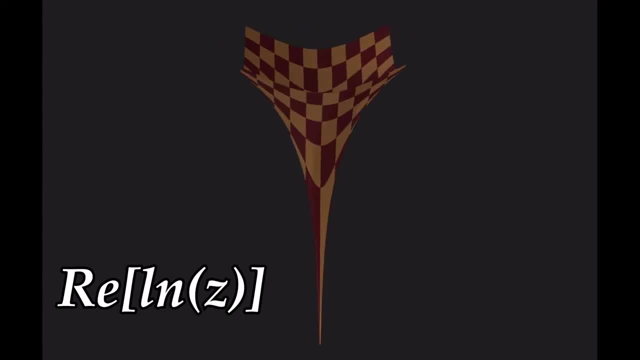 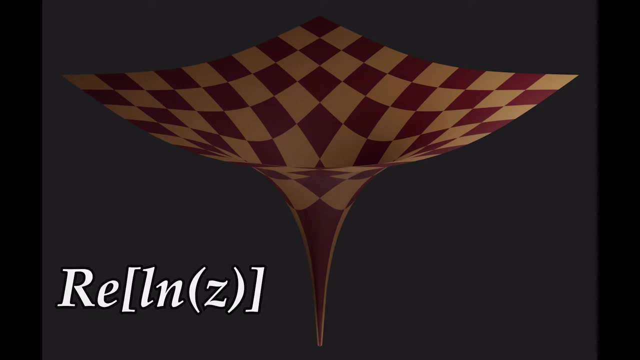 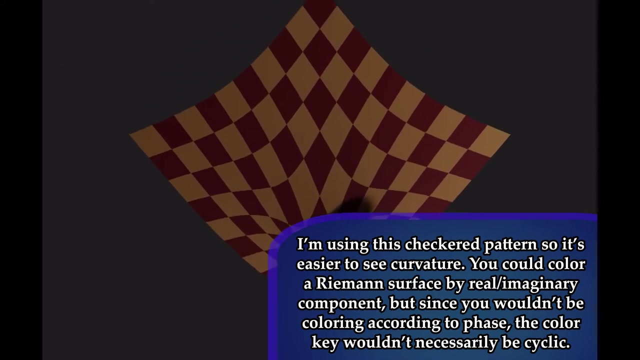 plane. the plot funnels down toward negative infinity. The funnel flattens out as we look farther away from the origin. Since the one shown here only depicts the real part of the function, we need a separate 3D surface for the imaginary. 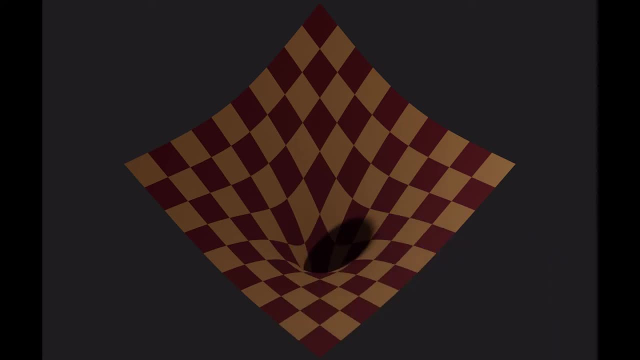 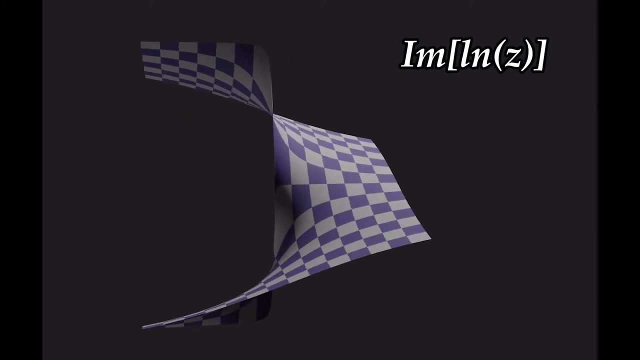 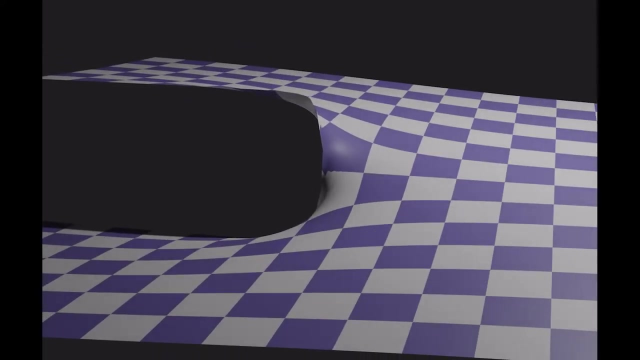 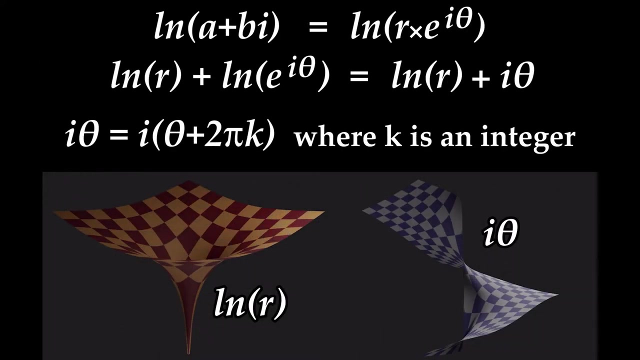 Then we imagine the imaginary component of the outputs. Using the third dimension for the imaginary component, we get this Again. looking farther from the origin, we can see the surface flatten out. Before moving on, there's something I want to explain. The complex natural logarithm has an infinite number of outputs for 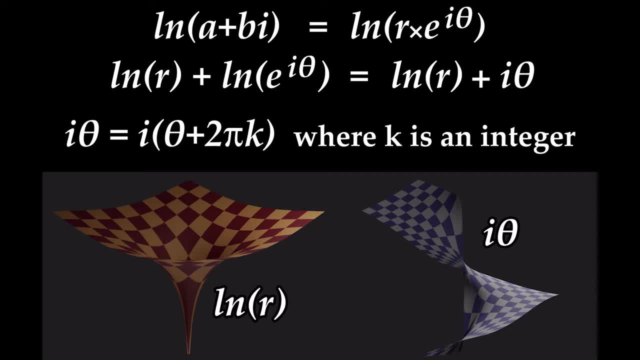 To understand the difference about these outputs, we need to think about them in polar form. If a complex number of the form r times e to the i theta is the natural logarithm of another complex number, then so is every other complex number of the same magnitude, with. 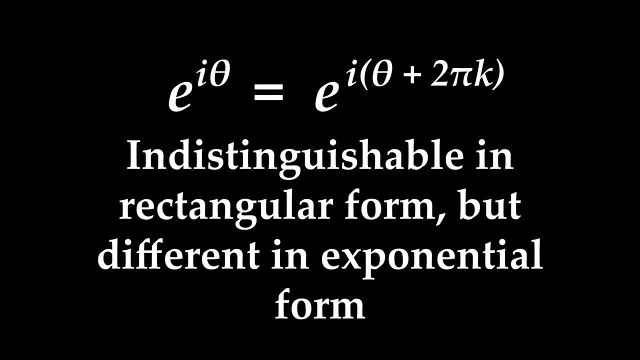 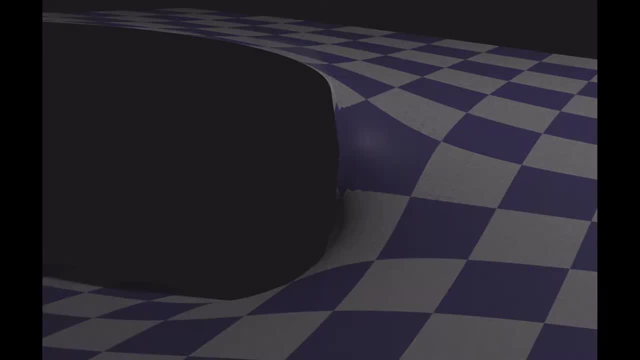 a phase that differs by some integer multiple of 2 pi. We can't describe these numbers as different in rectangular form, but we can in exponential form. What makes them different is the number of times they wind full circle in the plane. Going back to our plot, we see that when traveling up or down the surface we eventually reach. 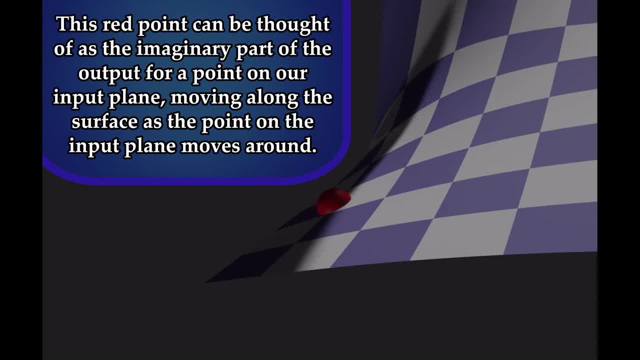 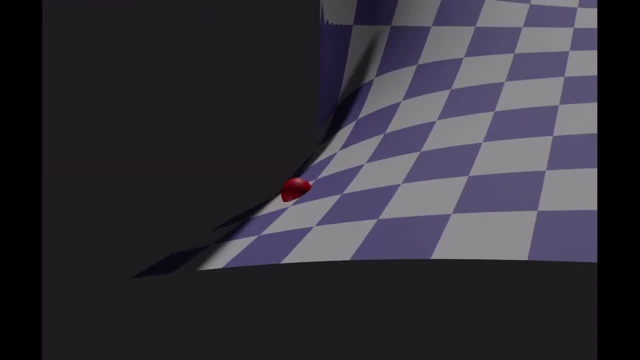 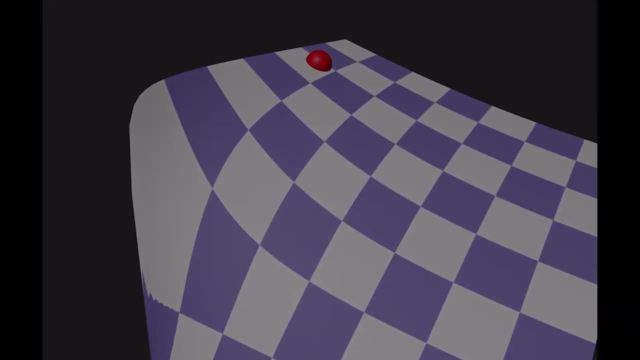 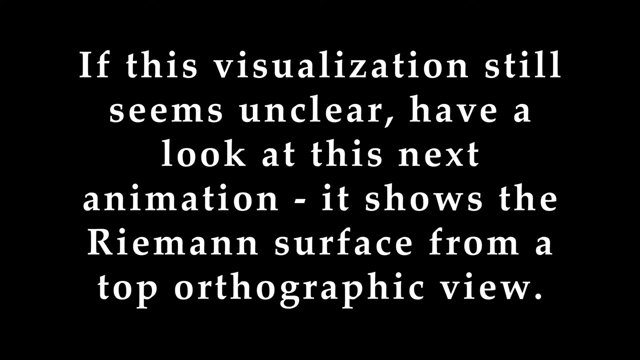 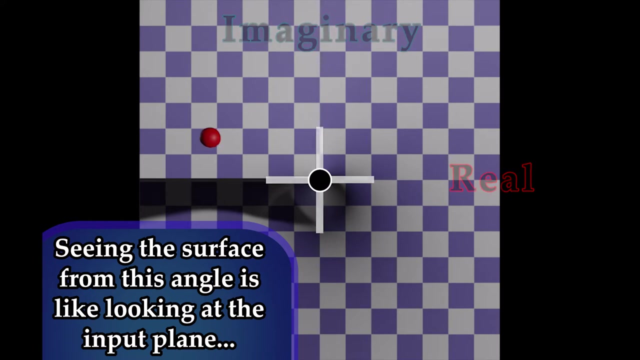 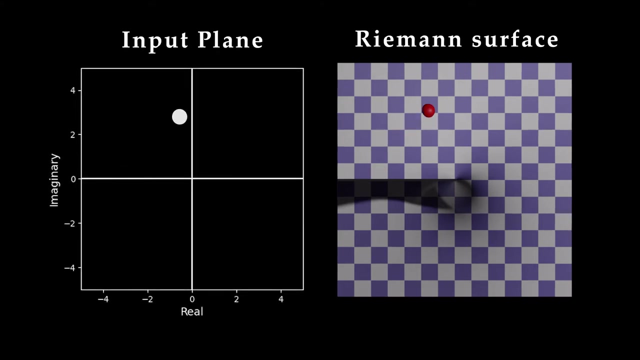 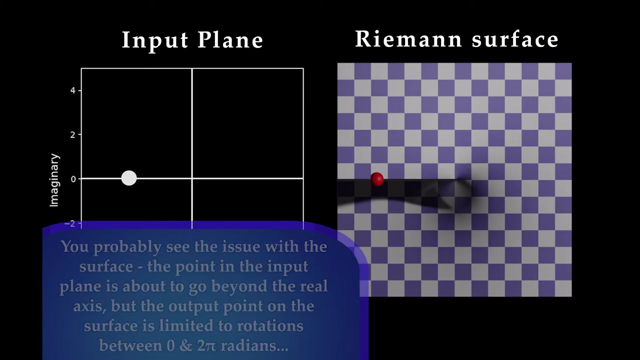 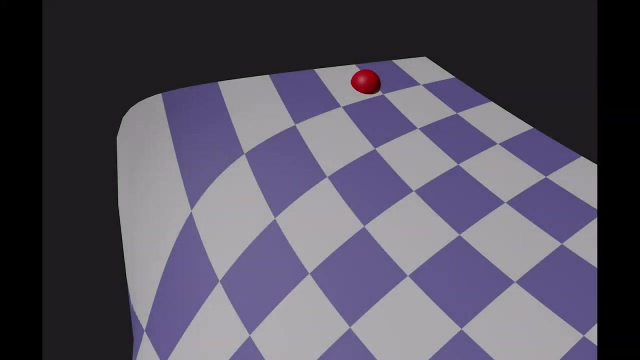 this discontinuity. at the edge, The red dot is the Mega Zaromite. Let's call it 1., 2., 3., 4., 5., 6.. It looks like this surface doesn't quite work, but since we know that there are an, 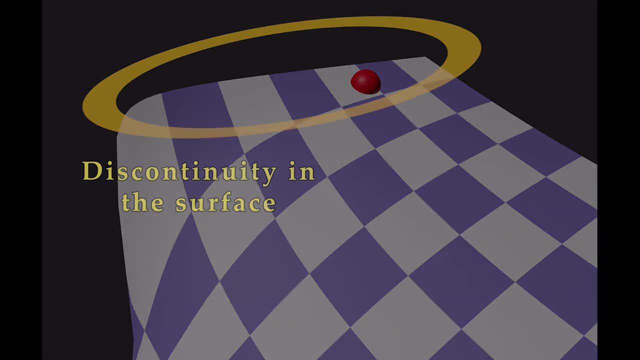 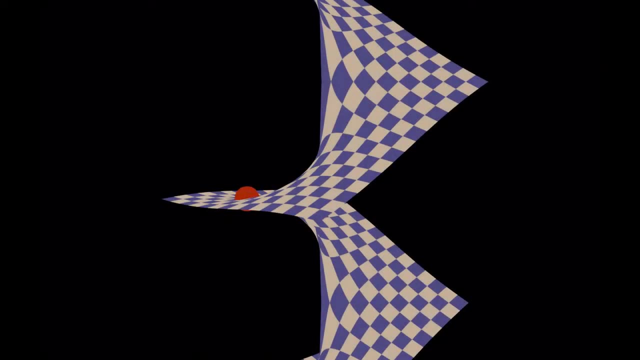 infinite number of outputs for the complex natural logarithm at each input. we can extend this particular plot by copying and pasting this single spiral an infinite number of times, connecting the top edge of one to the bottom edge of another. each time we do this, 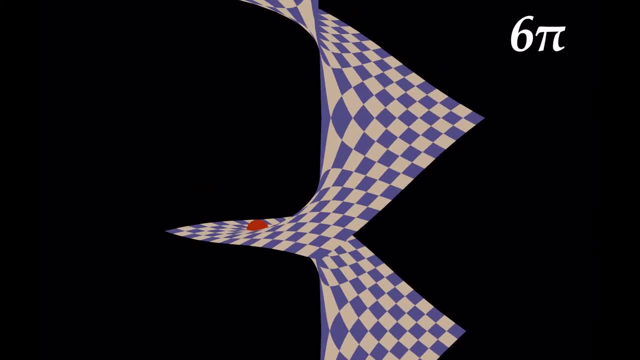 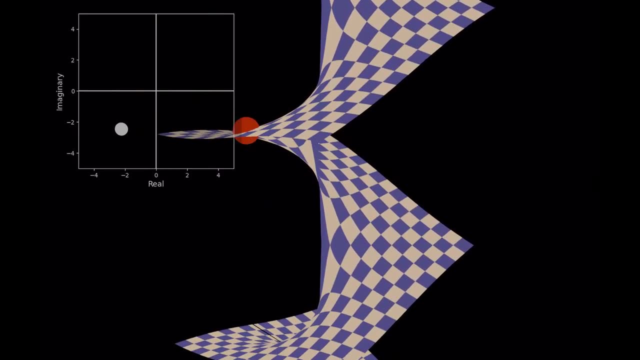 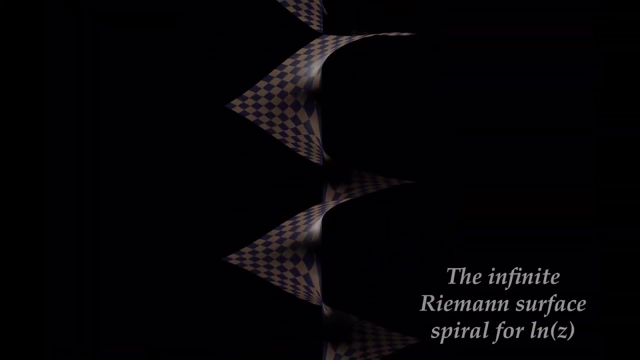 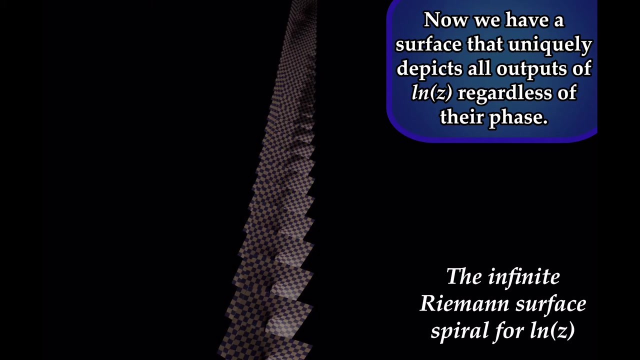 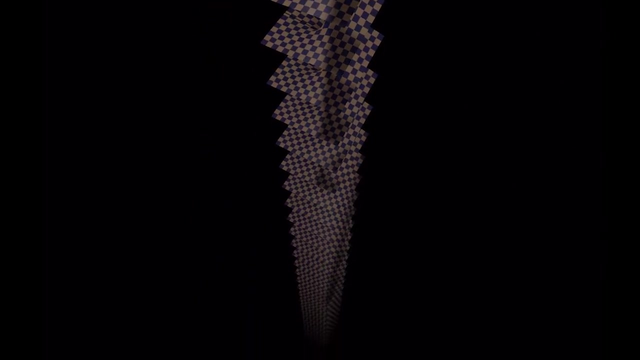 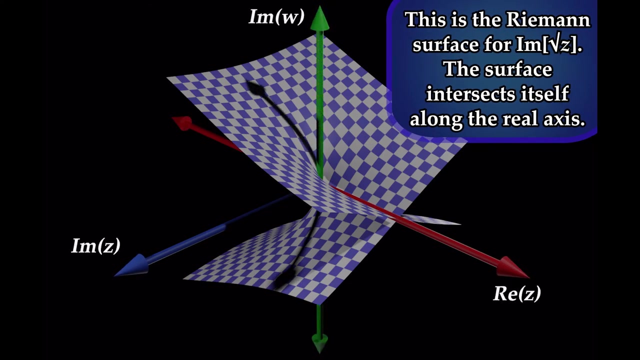 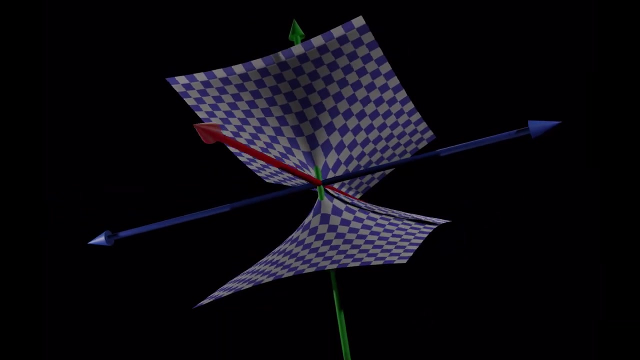 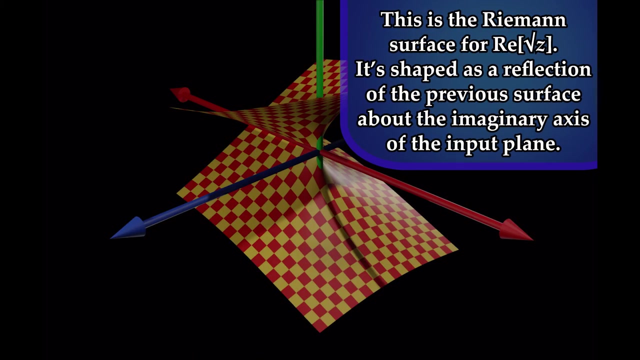 What we end up with is a continuous, infinitely ascending and descending spiral staircase that tells us not only the imaginary component of the output, but also how many times the number has wound around the origin of the complex plane. Now, what does the formula for theể and the resolution of the 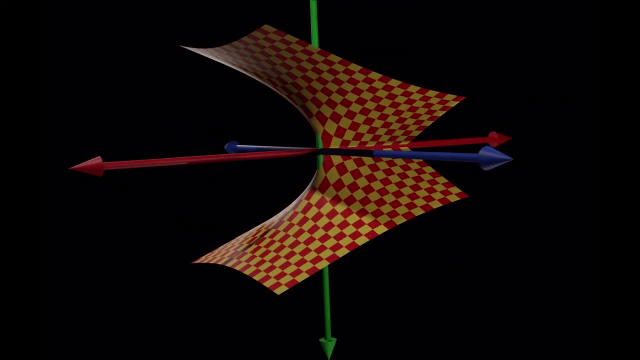 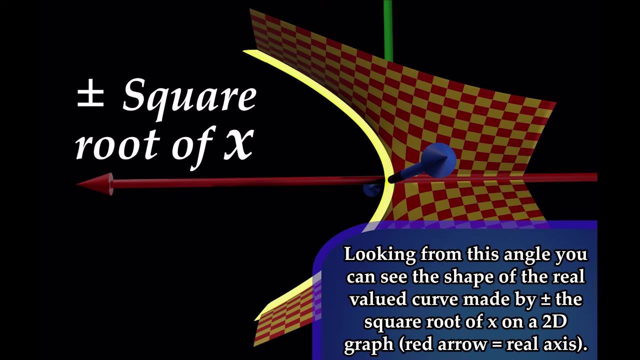 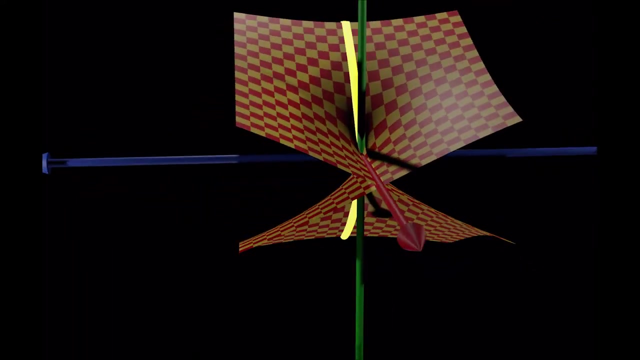 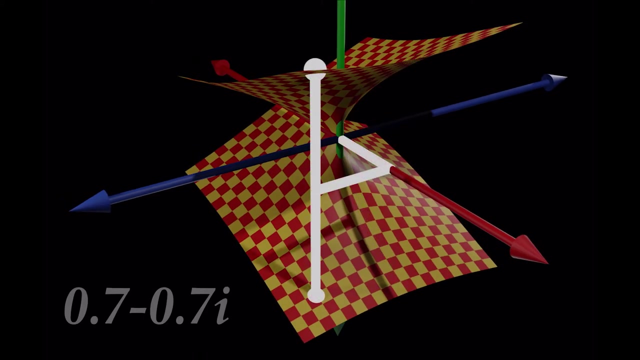 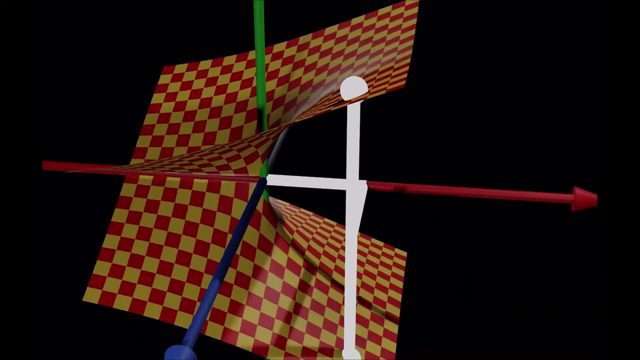 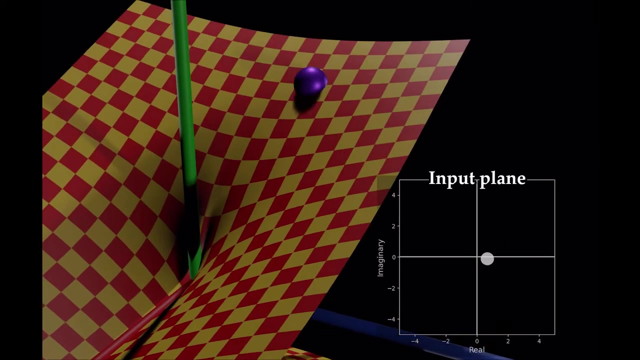 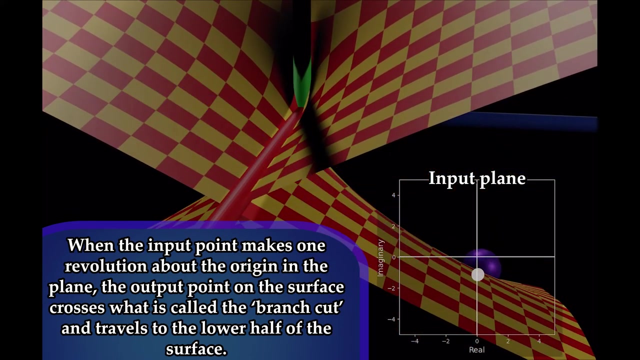 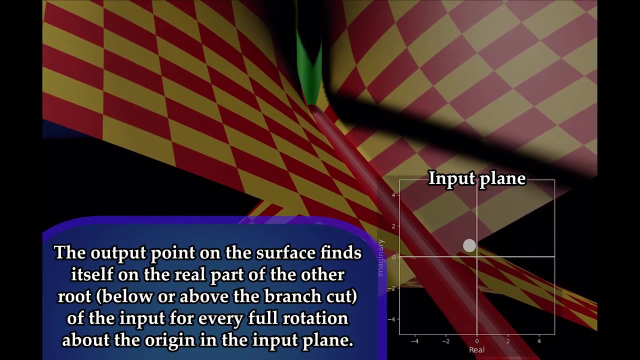 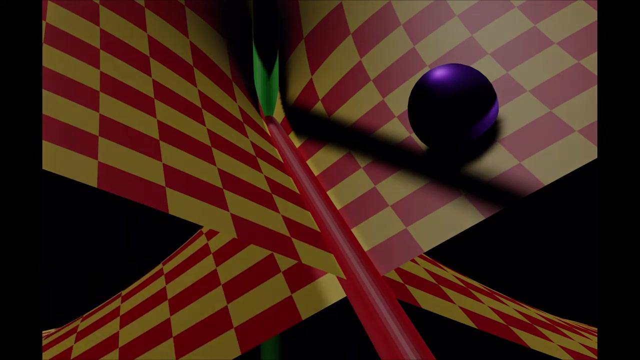 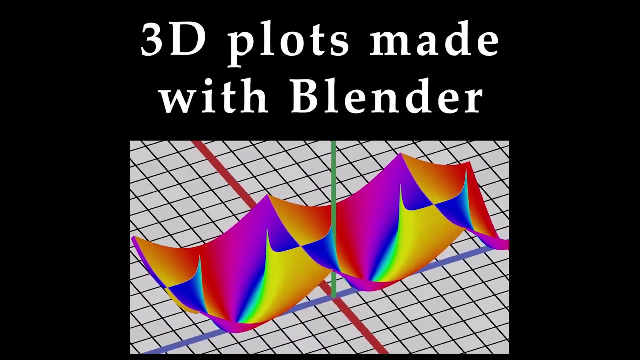 experiment. Let's find it out. Thank you, The three-dimensional plots in this video were made using Blender, a free, open-source 3D graphics software. 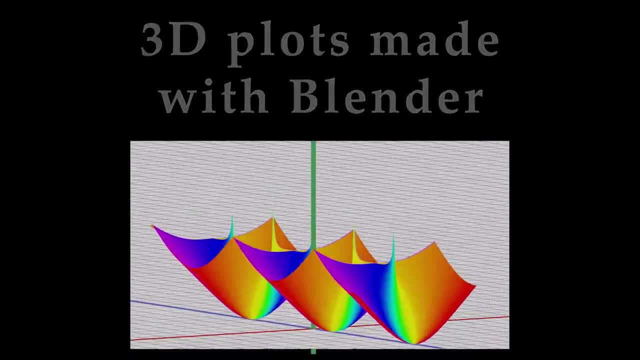 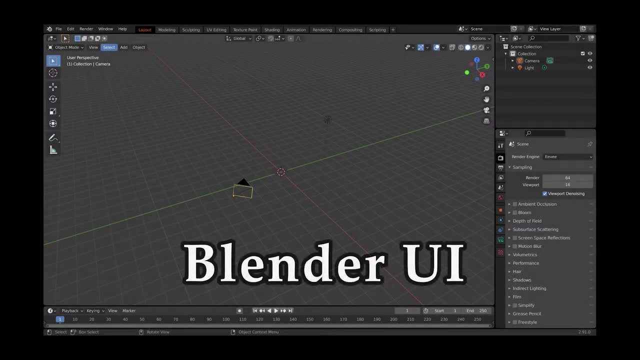 It's pretty amazing how far the software can go, considering it's free. In Blender, you can install what are called add-ons- extra scripts that enable you to do more things. So what I've tried doing is making a few small add-ons that allow you to plot complex, valued functions. 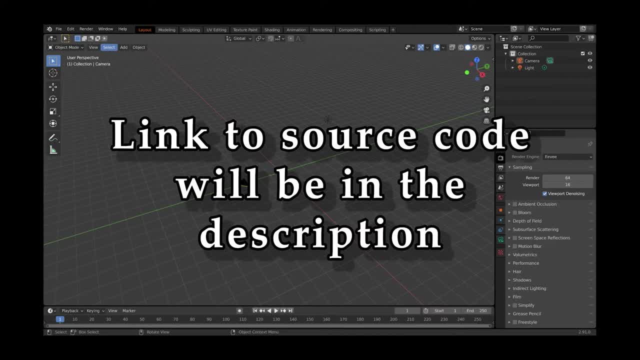 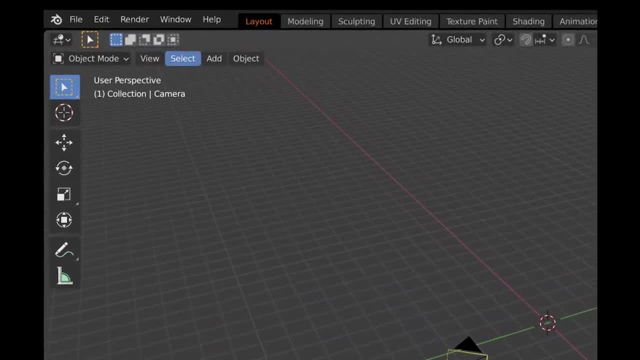 First, you can head to the GitHub page where the code is located. Simply download the Python files from here and save them to any folder you want. Once Blender is open, the next thing to do is click Edit in the top left corner, then Preferences, which will open a small window. 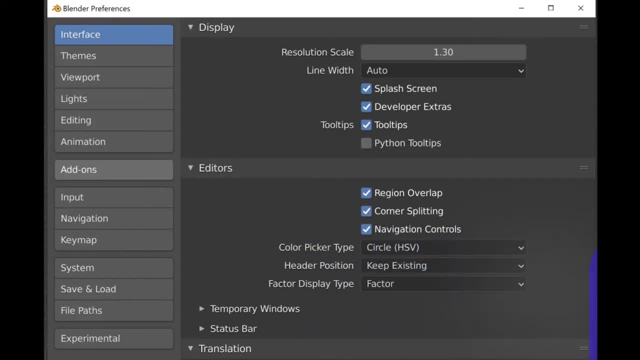 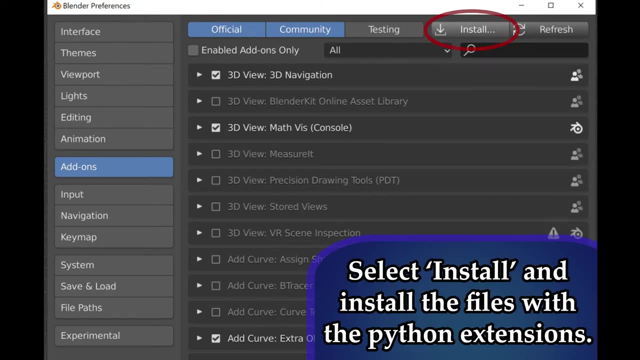 In the Preferences window, click Add-ons, then click Install around the top right-hand corner. This will bring up a file search window. From there, simply find the Python files from earlier and click on them to install them Now when you search for Modular Surface or Remon Surface.